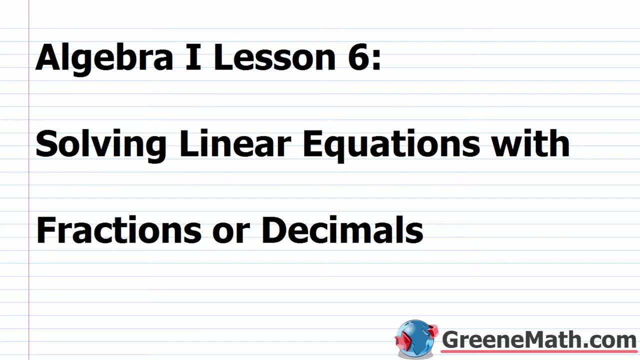 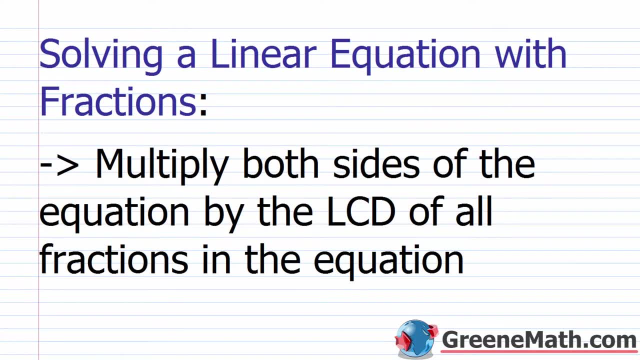 Hello and welcome to Algebra 1, Lesson 6.. In this video we're going to learn about solving linear equations with fractions or decimals. So up to this point we really haven't worked a lot with equations that have fractions or decimals. I kind of did that to keep it very simple in the 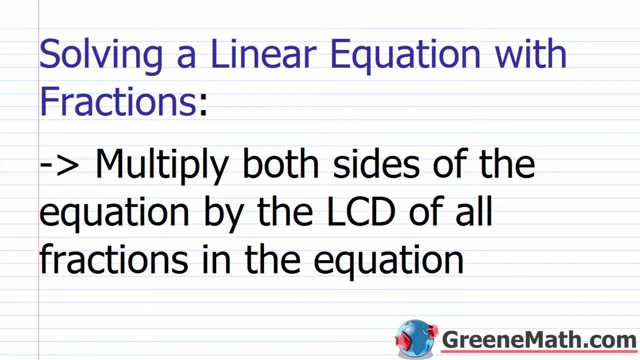 beginning. but as you kind of progress through your chapter on solving linear equations in one variable, you're going to see a lot of problems with fractions and decimals. So when they occur we can use a special trick to get rid of them. So let's first talk about how to solve a linear 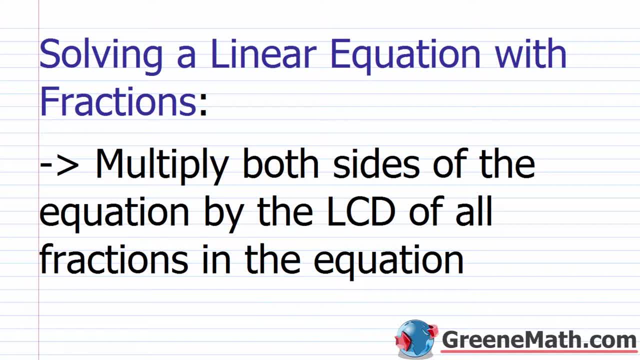 equation with fractions. Now, a lot of people hate fractions, so when they occur inside of an equation and you're just starting to learn equations, it makes it that much worse, right? You're already struggling to figure out how to solve an equation, and now I'm throwing fractions in there and you're 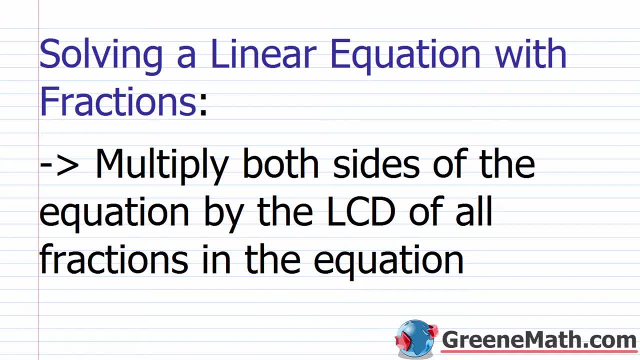 like: oh, what am I going to do? When you first start out the problem? you're going to clear your fractions by multiplying both sides of the equation by the LCD. Remember that's called the least common denominator of all fractions in the equation. So, for example, 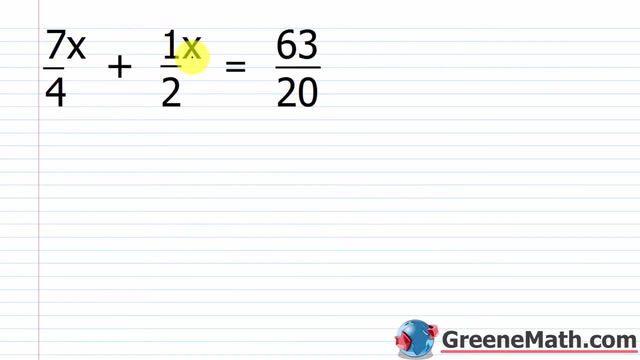 we have seven-fourths x plus one-half x equals 63 over 20.. What you'll do is look at all your fractions. so here's a fraction, here's a fraction, here's a fraction. Okay, I want you to look at the denominators of each fraction. so you have a four, you have a two and you have a 20. So four, two, three. 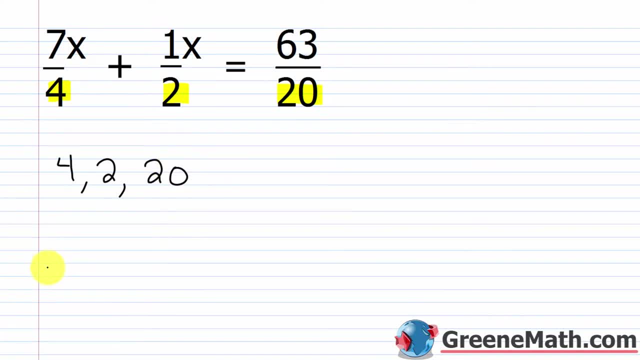 and 20, those are my denominators, and we want the LCD. remember the LCD is equal to the LCM, the least common multiple of the denominators. so what is the LCM of 4, 2 and 20? well, remember from pre-algebra the way we figure this out: we. 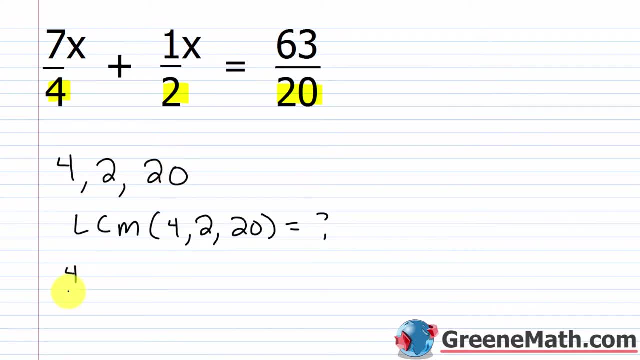 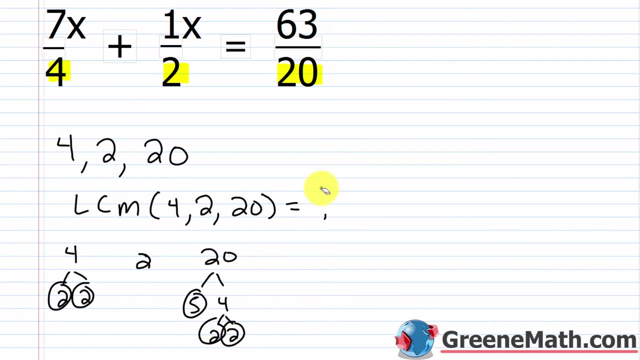 would factor each number. so 4 would be, 4 would be 2 times 2. 2 is a prime number that's not going to factor, and 20 is going to be 5 times 4. 4 is 2 times 2. very, very easy to do and to build the LCM: we take each prime number from each. 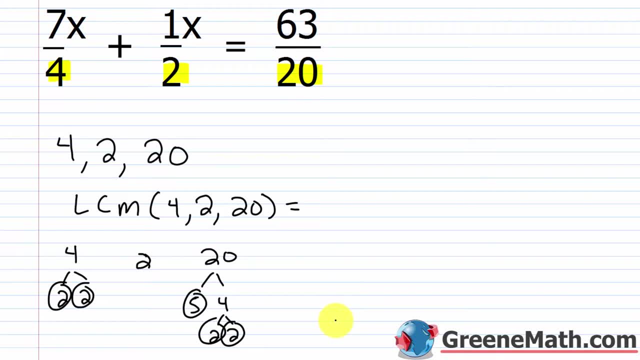 prime factorization and we throw it in there. the only thing is that you have to remember if a prime factor is repeated. so in other words, in four we have two factors of two, in two we just have that number, and in 20 we have two factors of two. i put the largest number of repeats between all of the 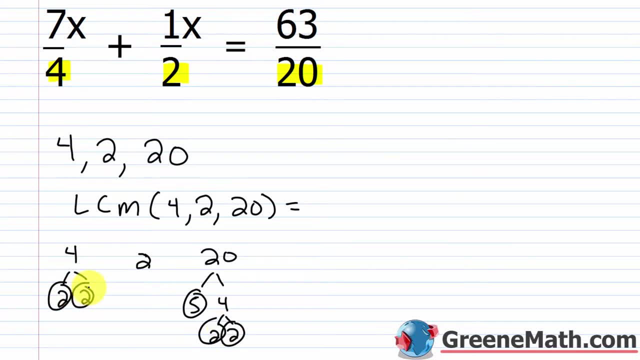 prime factorizations. so with the number two, it occurs twice at most, right, it occurs twice here, it occurs twice here. so i'm going to put two in when i build my lcm and if that doesn't make any sense to you, go back to the pre-algebra lesson on finding the least common multiple, and it will. 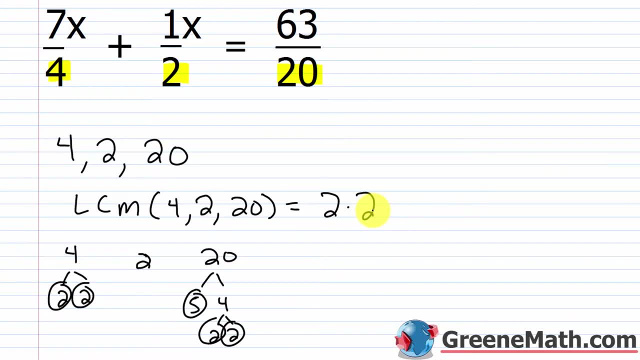 make sense to you, then all right now the next thing i want to put in here. i have a two and a two. i have a two here, a two and a two here. i only have a five left to put in. so throw in a five and two times two is four. four times five is 20. so the lcm for four, two and 20 is 20. 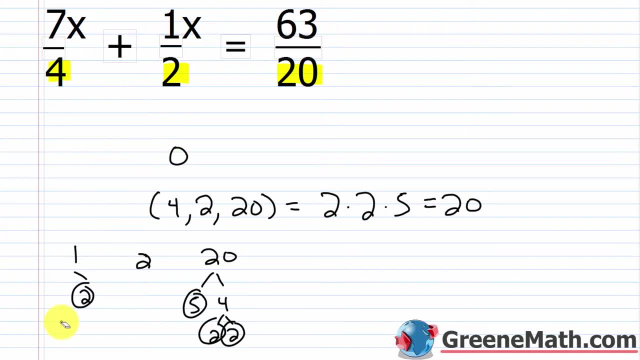 so that means my least common denominator here is 20. now, once i have figured that out, you all i do is multiply both sides of the equation by that and the fractions will go away. so i'll have 20 times seven. fourths x plus one half x equals 63 over 20 times 20. now, remember this is. 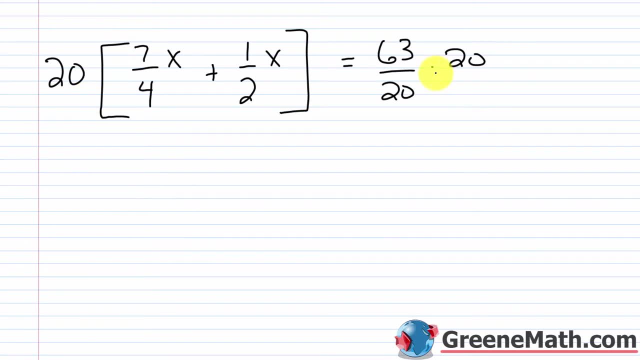 legal because of the multiplication property of equality. i can multiply both sides of an equation by the same non-zero number and preserve the solution. so on the right, it's pretty easy. this just cancels with this and i just get the number 63.. on the left, i've got to use my distributive. 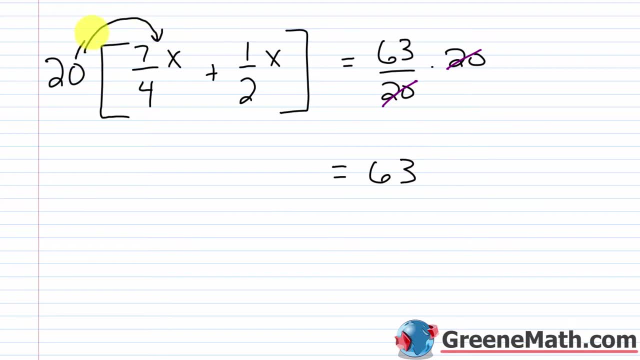 property and i've got to distribute 20 to each term here. so i'm going to end up with 20 times seven fourths x. so 20 times seven fourths x plus 20 times one half x, now you can look at c. okay, between 20 and seven fourths. this is going to cancel with this and give me five, five. 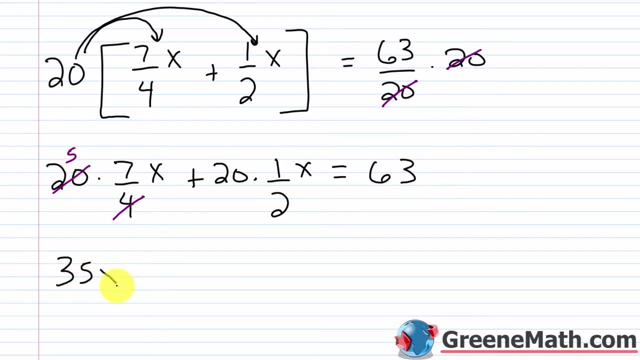 times seven is 35, so i'm going to have 35 x plus and then, over here, this is going to cancel with this and give me a 10 10 times one is just still 10, then times x, so i'm going to have 10 x there. 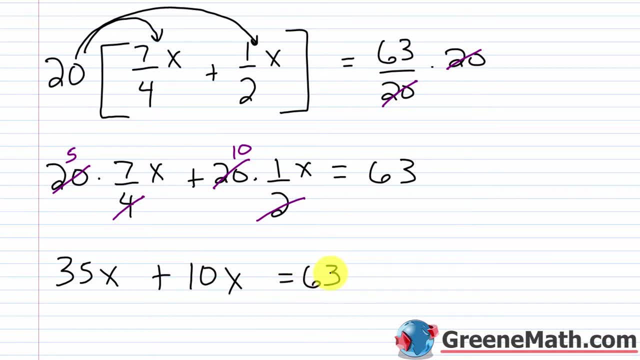 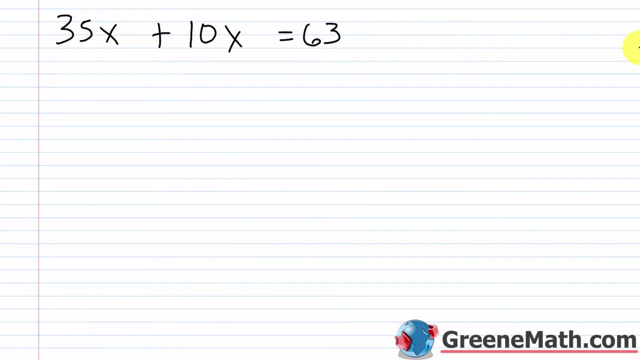 this equals 63, and we'll scroll down a little bit more. so now i have an equation that's clear of fractions and the solution is going to be the same as if i had just worked with the fractions. so i would start out by just combining like terms: 35 x plus 10 x is 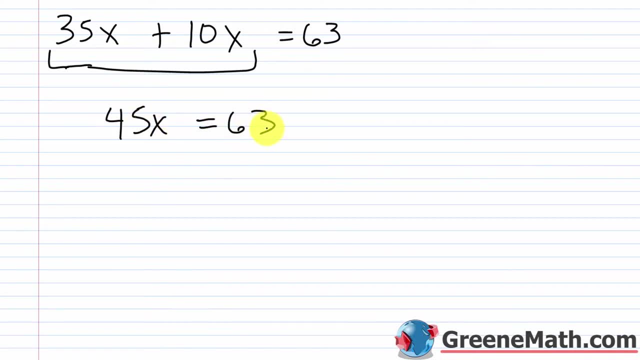 45 x and this equals 63. now to get x by itself, i divide both sides of the equation by the coefficient of x, which is 45. this will cancel with this and just give me an x and 63 over 45. that's not going to be a whole number. 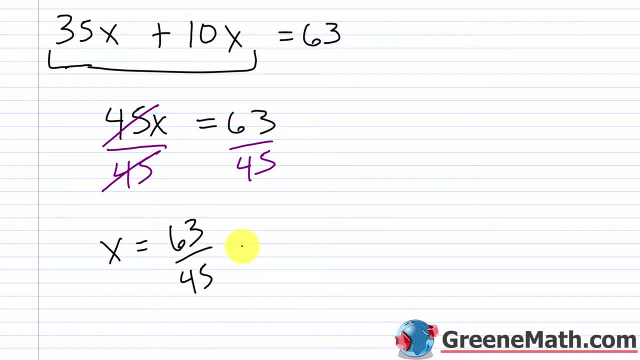 so i just have to reduce the fraction. so 63 is 9 times 7, 45 is 9 times 5, so the greatest common factor there is going to be not- i can cancel this with this and i'll have seven fifths right. so x equals seven fifths. you're going to get a lot of fractional solutions. 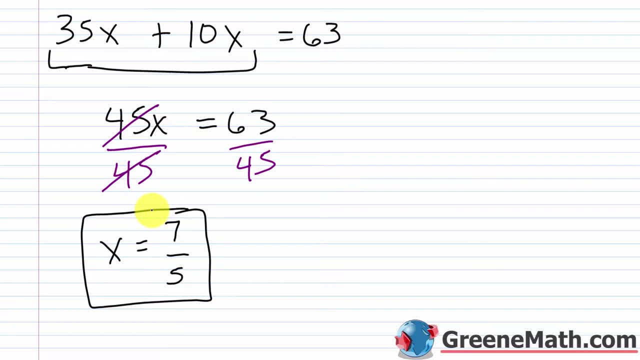 moving forward. i kind of stayed away from it in the beginning because i wanted to make everything nice and easy for you to understand before we start really ramping it up and dealing with fractions and decimals. all right, so i want to do two things. i want to check this, so let's erase 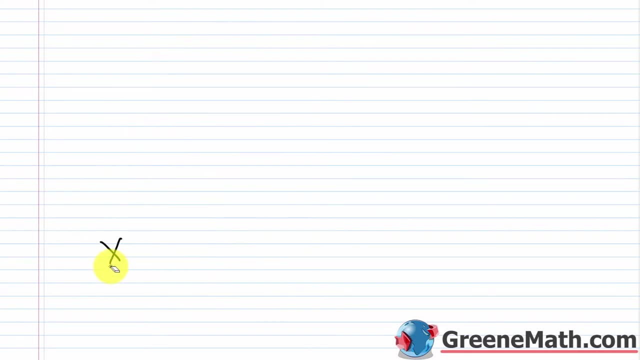 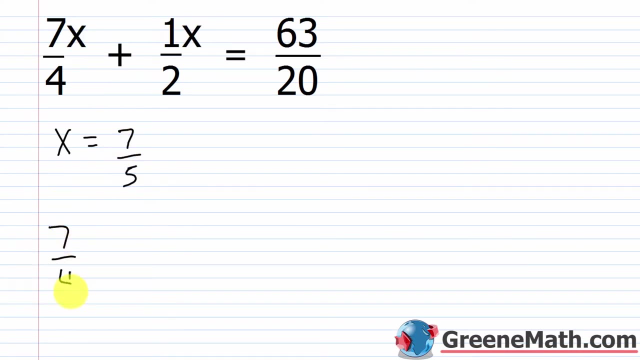 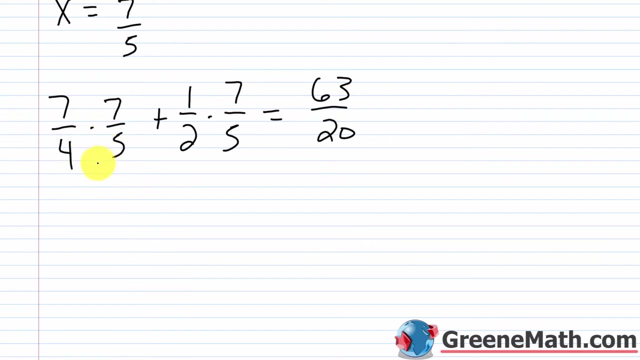 everything here and we're going to go back up to the top. so remember: x equals seven fifths, so i'm going to plug a seven fifths in. everywhere i see an x. so seven fourths times seven fifths plus one half times seven fifths equals 63 over 20. all right, so over here nothing i can cross. cancel, so seven. 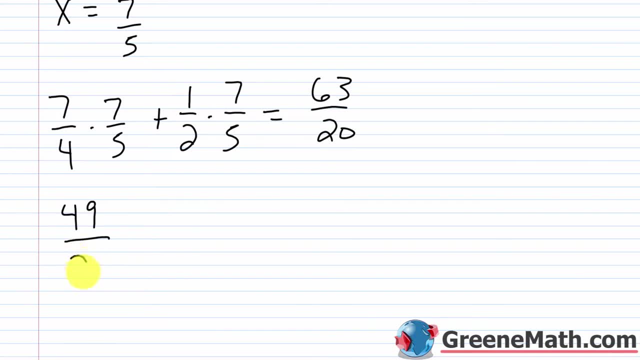 times seven is 49, and four times five is 20. plus over here, nothing i can cross cancel. one times seven is seven. over two times five, that's ten. now, in order to add, i've got to have a common denominator, so i'm going to go ahead and just multiply this by two over two. 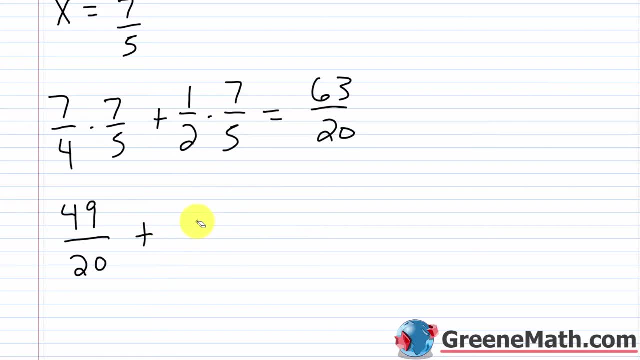 and this will be 14 over 20, 14 over 20 and this equals 63 over 20 and, of course, the left and the right side are going to be equal. 49 plus 14 is 63. this is over 20, and this is equal to 63 over 20. 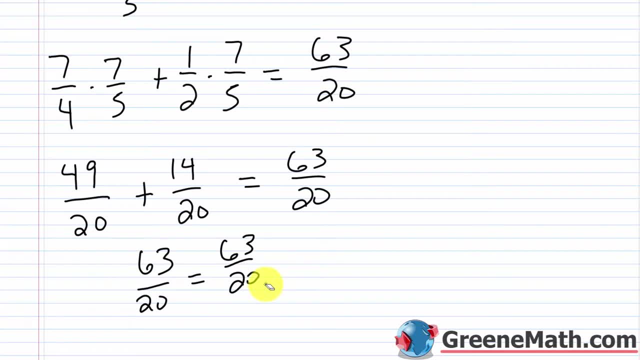 so our solution, x equals seven fifths, is correct. one thing i want to show you: if we would have just left the fractions as is and just work with them, you're going to get the same answer. so clearing the fractions is just more of a trick that you can use if you just don't like. 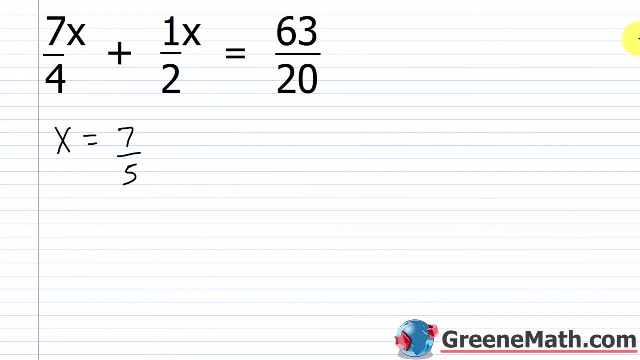 working with fractions. sometimes it just makes it a lot easier. right, nice and simple. so let's say i have seven fourths. seven fourths x plus one half x equals 63 over 20. if i want to, i can combine like terms here to simplify on the left. so move this kind of x over to the side and get a common. 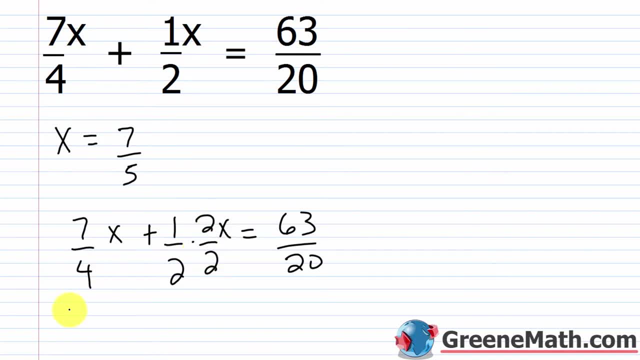 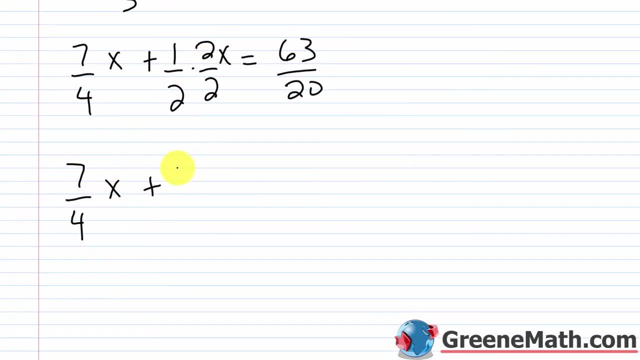 denominator. multiply this by two over two, so then i'll have seven fourths. let me scroll down here. i'll have seven fourths x plus one times two is two, so two over two times two is four, so two fourths x equals 63 over 20. so to combine like terms here i'm just going to add the numerator seven plus. 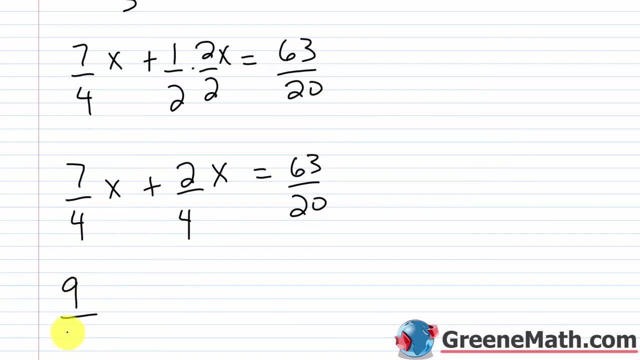 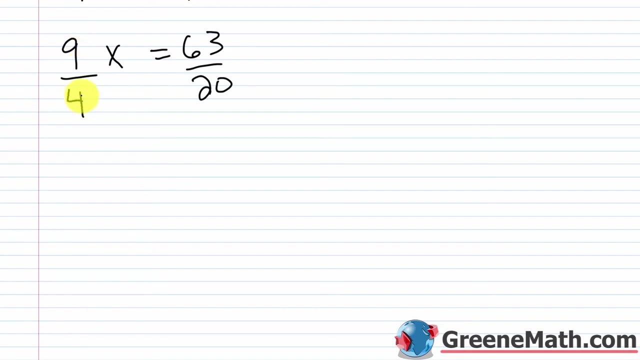 two is nine, so i would have nine. the common denominator is four, so nine fourths. then times x. now how do i isolate the variable here we talked about in one of our beginning lessons? if i have a fractional coefficient for x and i want x by itself, remember, if i multiply a number, 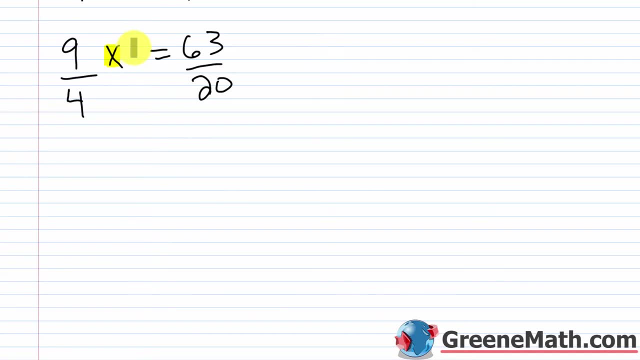 by its reciprocal, the result is one. so if i multiply nine fourths by four ninths, remember the reciprocal is found by taking the denominator and putting it into the numerator. taking the numerator and putting it into the denominator, i'm going to get one right if i multiply these two. so 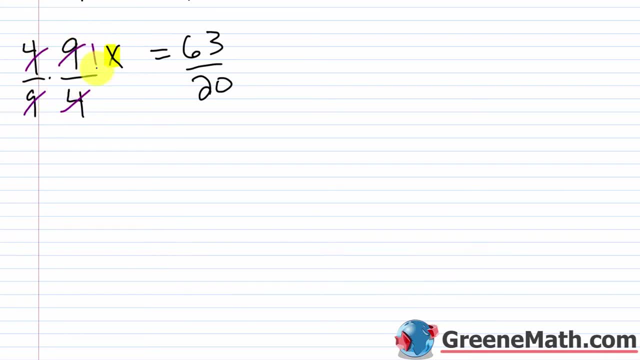 this, this, this, that all cancels. so this is one x now, because i do it over here. i've got to do it over here. so this cancels with this and gives me seven. this cancels with this and gives me five. so what am i going to have? i'm going to have x equals seven fifths, and that's exactly what we got by. 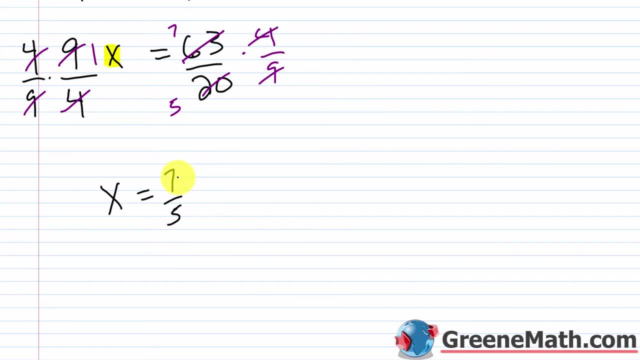 clearing the fractions now in this particular case, because i'm very good at working with fractions, right, i've been doing a long time. it didn't take me any longer to work this problem with the fractions involved for yourself. you might not be that good with fractions, so you might want to just. 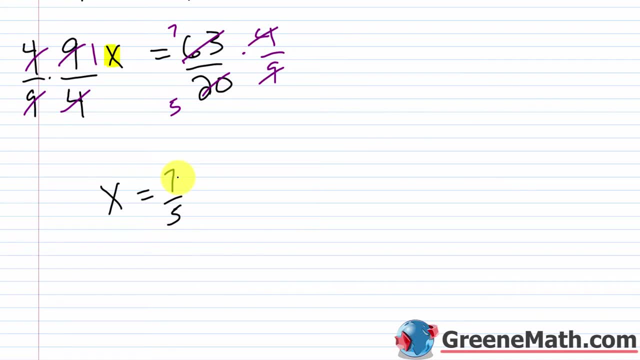 take the time and clear the fractions, so that you don't have the added stress of trying to solve an equation and trying to work with the fractions together. now, when we get to decimals, because most of you work with calculators- you might not want to clear it. it might not save you any time, it just. 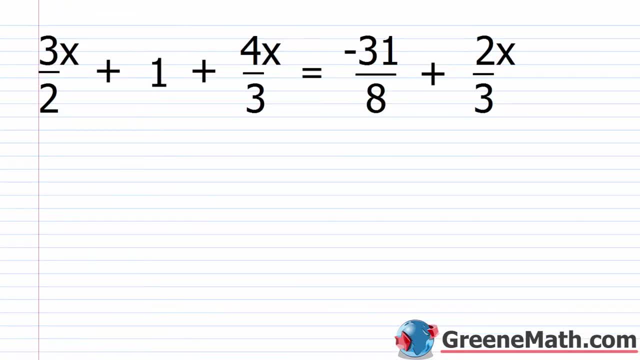 depends. all right, let's take a look at another one. so we have three halves x plus one plus four thirds x equals negative 31 eighths plus two thirds x. all right, so what i'm going to do is again clear the fractions from the equation. so let's look at our denominators. we have a two, a three, an eight and a three. now i'm 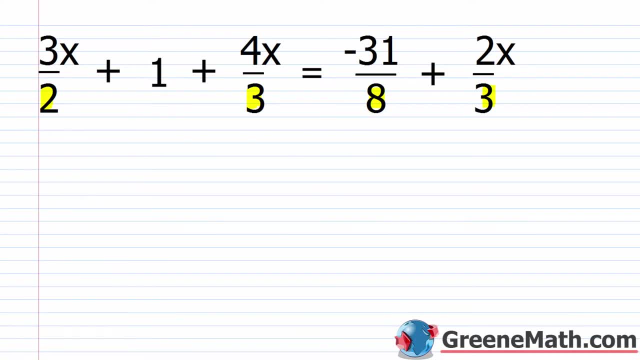 looking for the lcd, the least common denominator and the way i find that i want the least common multiple of the denominator. so two, three, three and eight, and i'm not going to put three in twice. right, it's the same number. so two doesn't factor, so i'm just going to throw that in there. three doesn't factor, just going to throw that in. 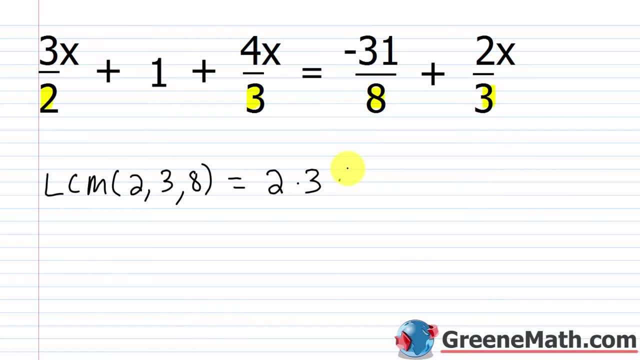 there, and eight is three factors of two. so how many factors of two am i going to put in when i'm building my lcm? only three, right. so i'm going to put one and then twos, because i already have one over here from when i did this. remember, when you build your lcm, you want the largest number of 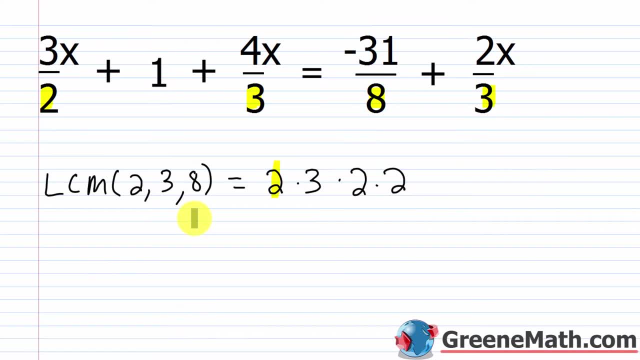 repeats between any of the prime factors and you want the largest number of repeats between any of the prime factorizations. so between eight, you have one, two, three and two. you have one. the largest number of repeats is three. so three goes in when you build this. okay, so we have two times three. 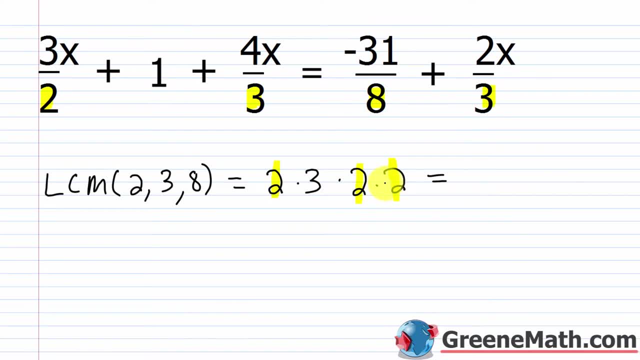 which is six times two, which is twelve times two again, which is twenty four. so that's going to be my lcm for those numbers, and so my least common denominator is twenty four. all right, so lcd is equal to twenty four, and so i multiply twenty four by both sides of the equation, so i'm 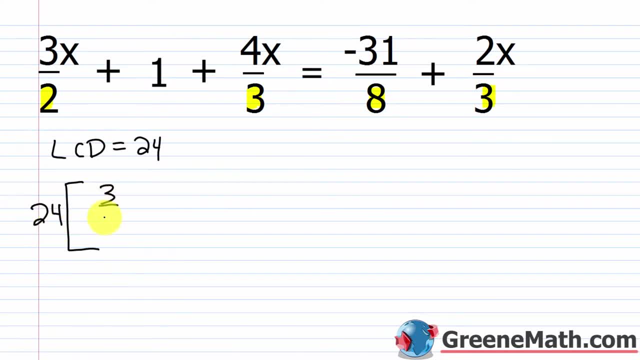 going to put some brackets here. very important that you use brackets or parentheses because you need to distribute. okay, you need to distribute this value of twenty four to each term. i see a lot of students will just write twenty four next to this and then they multiply by that and then 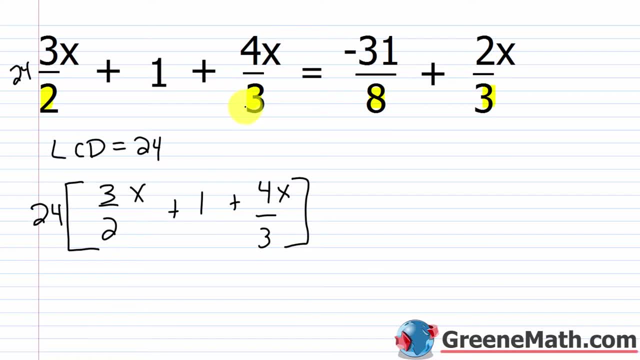 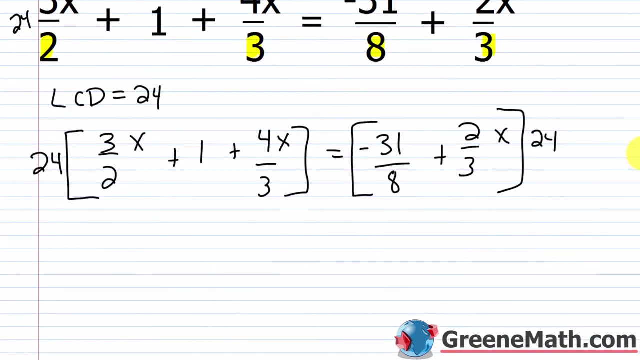 they're done. that's, you need to multiply twenty four by every term to make this legal. okay, so over here, negative thirty one eighths plus two-thirds x, and we'll enclose this inside some brackets as well, and then we'll use our distributive property. so what i'm? 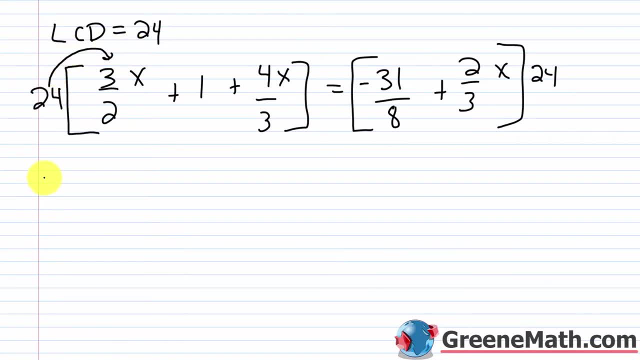 going to do? i'm going to multiply twenty four by three halves x, so twenty four times three halves x, and as i do it i'm just going to do the calculation kind of save some time. so twenty four would cancel with two and give me twelve. twelve times three is thirty six, so this would 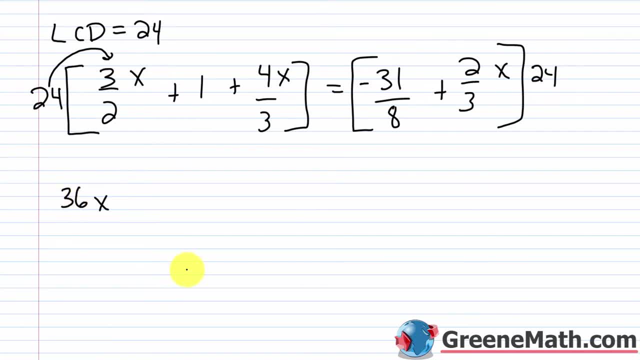 be thirty six x. this is thirty six x, okay, plus next i'd have twenty four times one. that's very simple. that's just twenty four. then, plus next i'd have twenty four times four-thirds x. so twenty four times four-thirds x. the twenty four would cancel with the three and give me an eight, eight times. 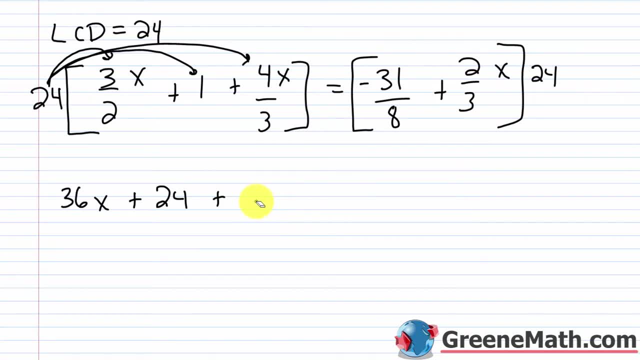 four is thirty two, so this would be thirty two x, thirty two x. and then this equals- i'm going to do the same thing over here- so twenty four times negative thirty one, eighths. so negative thirty one eighths times twenty four. this cancels with this and gives me a three, three times negative thirty. 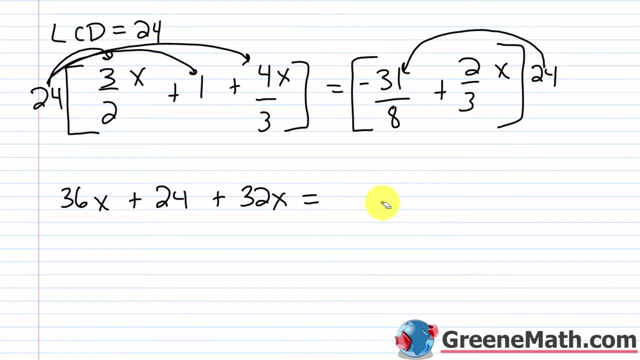 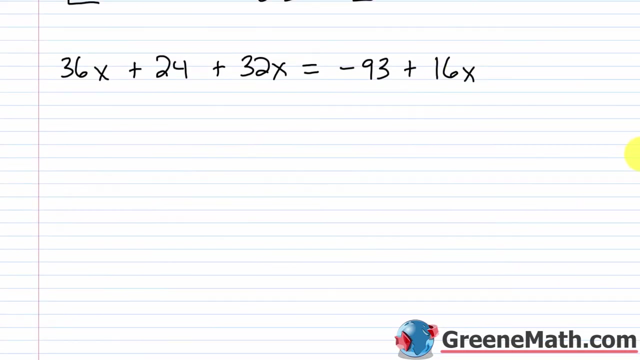 one is negative ninety three, so negative ninety three. and then i have one more twenty four times two-thirds x. so that's going to be plus two-thirds x times twenty four, and this twenty four we cancel with sixteen x. okay, so now we're free of fractions. now i just go about my usual business, which is to 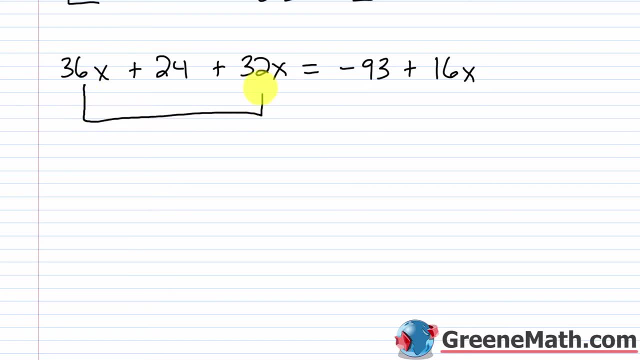 simplify the left and the right side. so this over here, thirty six x and thirty two x, we can combine like terms. that's going to give us sixty eight x. so sixty eight x plus twenty four equals. over here i really can't do anything. i just have negative ninety three plus sixteen x. 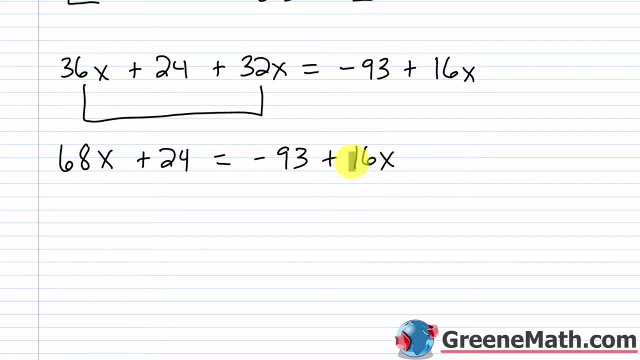 Now, as we learned in previous lessons, we've got to get the variable terms on one side of the equation. I have 16x over here and I have 68x over here, so I need to move one of them. I always move the one on the right to the left. I like my variable to end up on the left, so I'm going to. 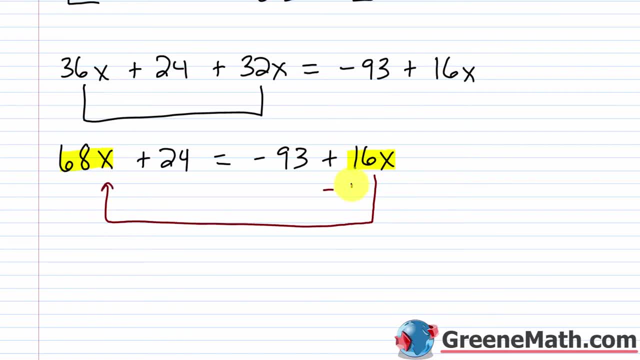 move this over here, and the way I'm going to do that, I'm just going to subtract 16x from both sides of the equation. That'll go away, and then minus 16x over here, 68 minus 16 is 52, so this: 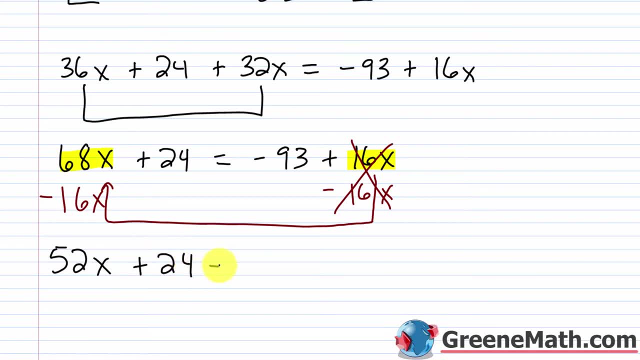 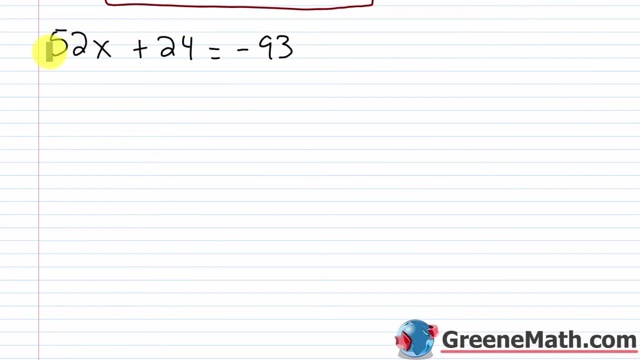 would be: 52x plus 24 equals negative 93. All right, so now I want to get the variable term by itself, and to get this by itself I need to subtract away 24. right, because I have plus 24 over here. that's next to the 52x, so minus 24. 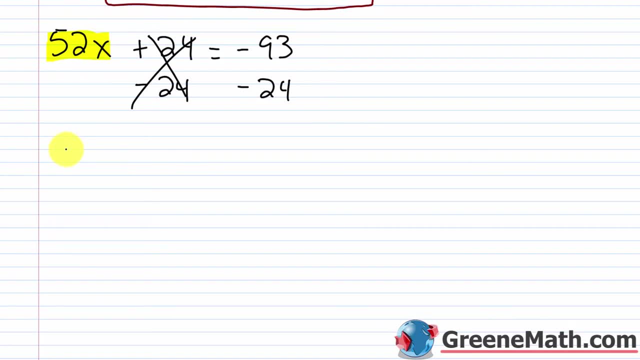 and I'm going to subtract away 24.. Minus 24, so that's going to go away. The left side is now just 52x, and on the right side, if I have negative 93 minus another 24, I'm going to end up with negative 117.. All right, the final. 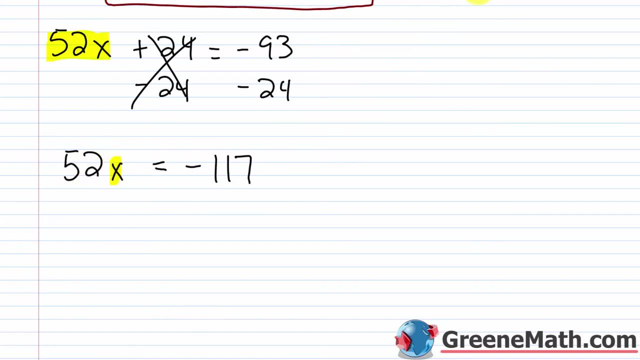 step here is to isolate the variable completely and if I look at it, I have what I have 52 times x. so to get x by itself, I divide by 52. I divide by that coefficient of x, All right, so divide both sides of the equation by 52.. 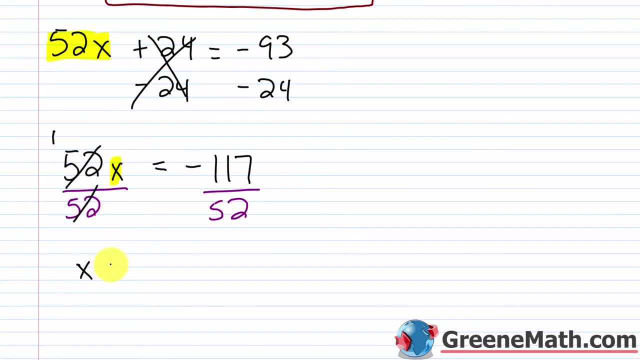 This will cancel. I'm going to take this and give me 1.. 1 times x is just x, so that's going to be equal to negative 117 divided by 52. So this won't result in an integer or whole number, so we're just going to reduce the. 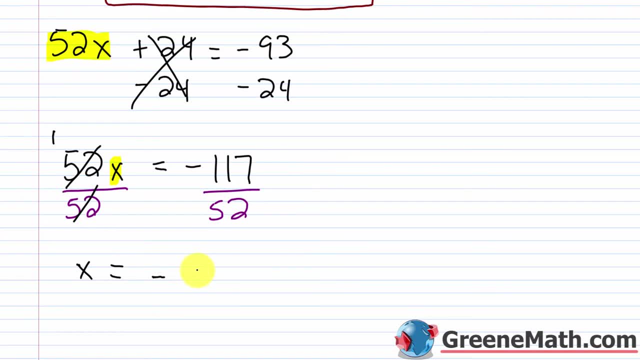 fraction. So negative 117, I'm going to write negative 1 times 13 times 3 times 3. and for 52, I'm going to write 13 times 2 times 2.. So what can I cancel? What can I cancel? I can cancel the. 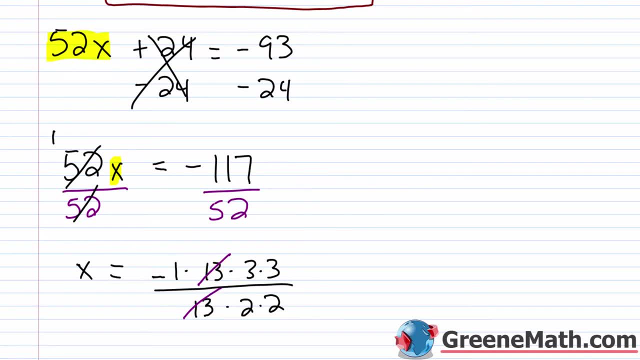 13 with this 13 and I'm really left with what. I'm left with negative 1 times 3 times 3, or negative 9 over 2 times 2 or 4.. So my answer here is going to be that x equals negative 9. fourths: 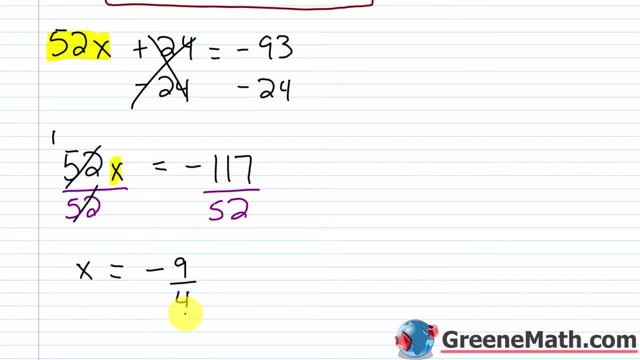 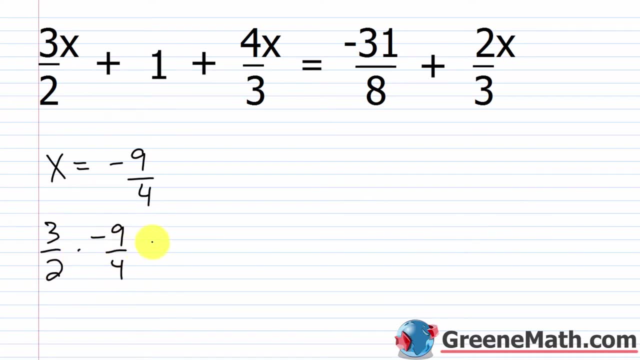 x equals negative 9 fourths. So I'm going to plug in a negative 9 fourths. everywhere I see an x, So I'm going to have three halves times negative 9 fourths plus 1 plus four thirds times negative 9. 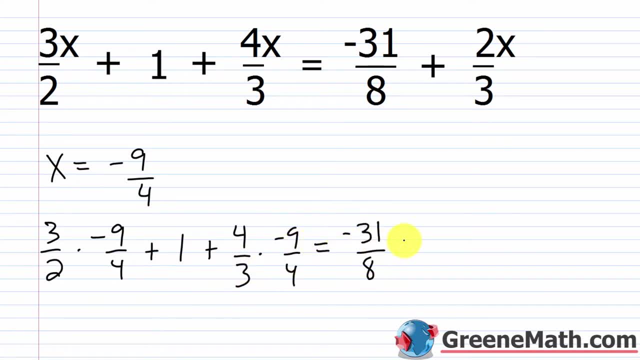 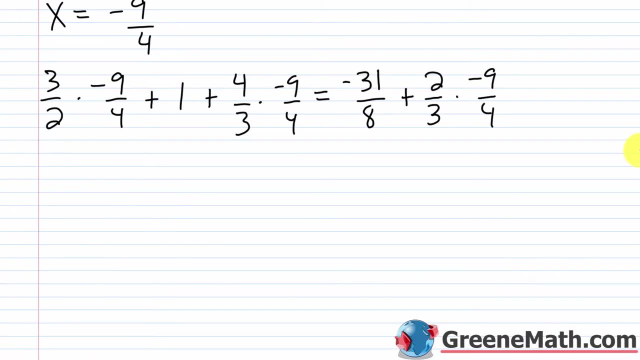 fourths is equal to negative 31 eighths plus 2 thirds times negative 9 fourths. All right, So if we have three halves times negative 9 fourths, what can we cancel? Well, nothing, So we just have to do. 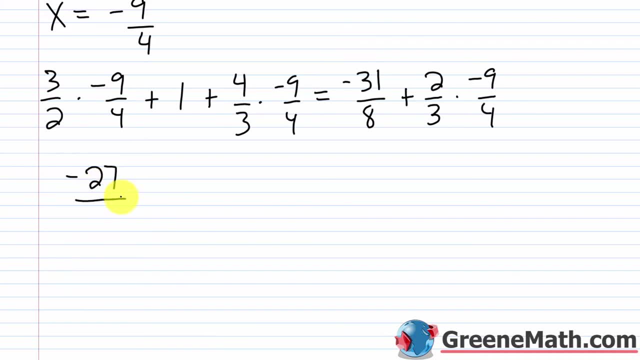 the multiplication 3 times negative, 9 is negative 27.. 2 times 4 is 8.. So then plus 1 plus over here, this 4 would cancel with this 4 and I'd have negative 9.. Thirds, Negative 9, thirds and equals, we have negative 31. eighths plus over here. I can cancel. 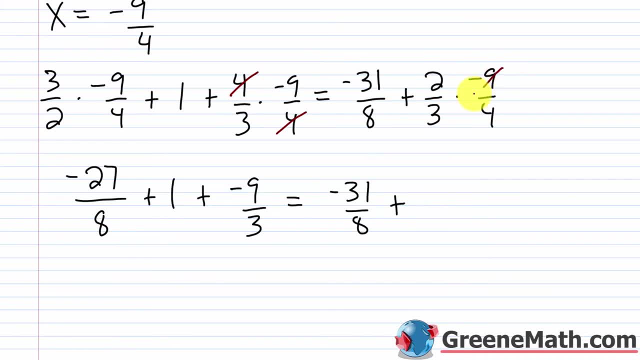 before I multiply: Negative 9 divided by 3 would be negative 3. So this cancels with this and gives me a 3. And this will cancel with this and give me a 2 down here. So this completely canceled out. 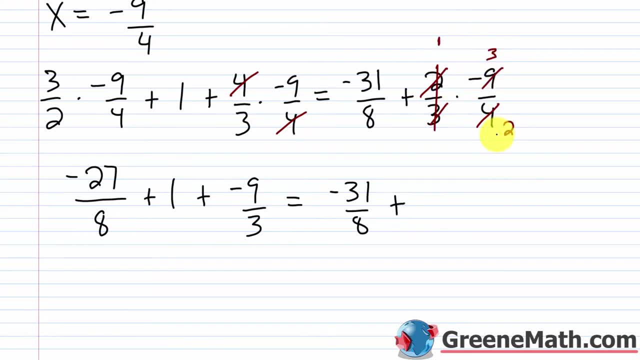 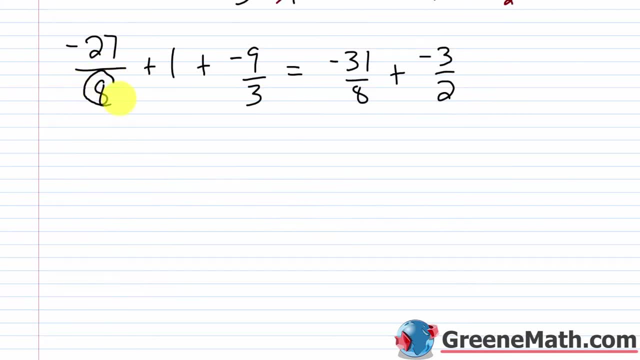 That's just a 1 now. So we'd have basically just negative 3 halves. So plus negative 3 halves, All right. So on the left, I got to think about getting a common denominator. So 8 is going to factor into 3 factors of 2.. 3 is not going to factor, So 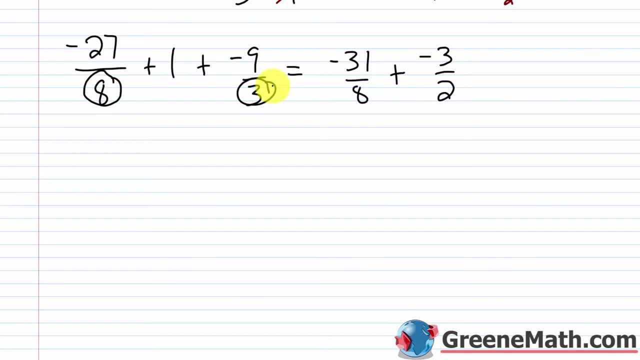 the best I can do there for my LCD is going to be 24.. Right 8 times 3.. So negative 27 over 8 times 3 over 3 plus for 1. I'm just going to write it as 24 over 24.. It's the same thing as 1.. 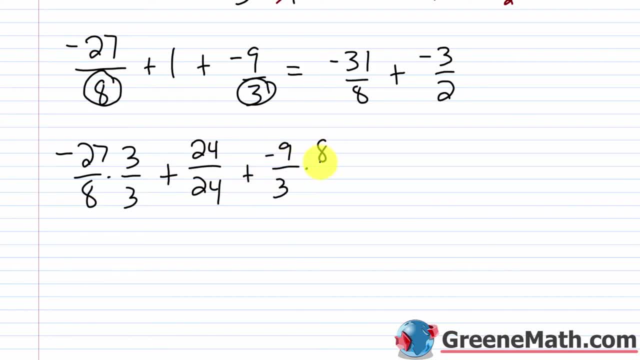 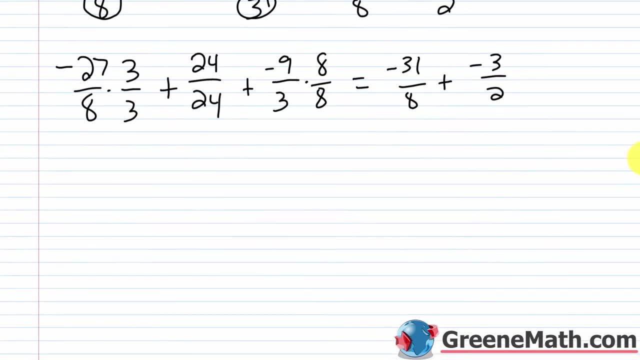 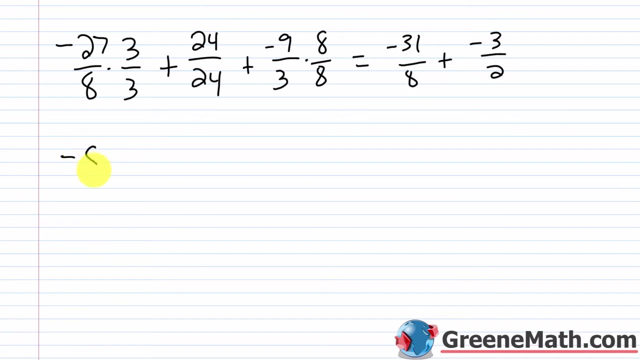 And then plus, we'll have negative 9 over 3 times 8 over 8.. Put this, equal to negative 31 eighths plus negative 3 halves. All right, So what is negative 27 times 3?? Well, that's negative 81. So this would be negative 81 over. 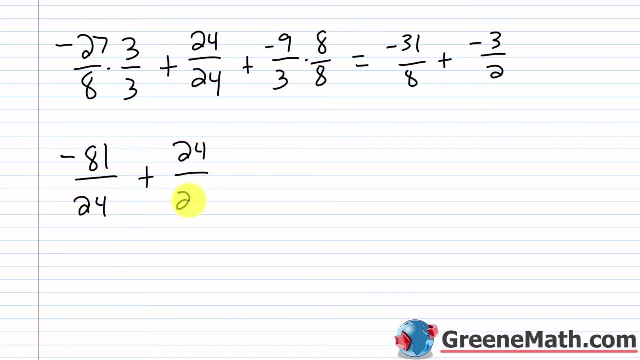 24 plus 24 over 24, plus negative 9 times 8 is negative 72 over 24.. Let's go ahead and figure this out real quick. So if I have negative 81 plus negative 72. So 81 plus 72, kind of mentally. 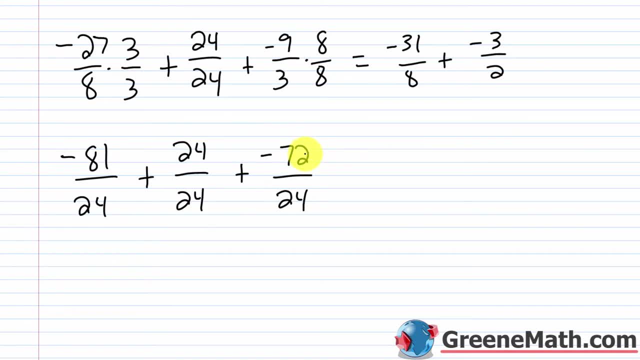 1 plus 2 is 3.. 8 plus 7 is 15.. So that'd be 153.. Attach the negative. So that's negative 153 plus 24.. And we can kind of do that in our head also, because really think about 153 minus 24.. That's going to give you 129. 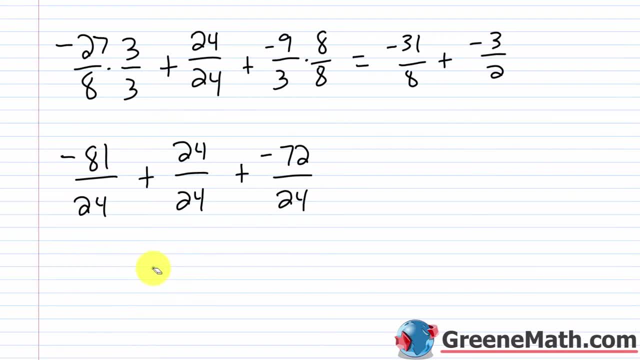 and then just slap the negative on there. So we would have negative negative 129 over 24.. So this is equal to: and then over here, really, I can easily see that the LCD is going to be 8. So I just want to make sure that I have that right. So I'm going to go ahead and do that. 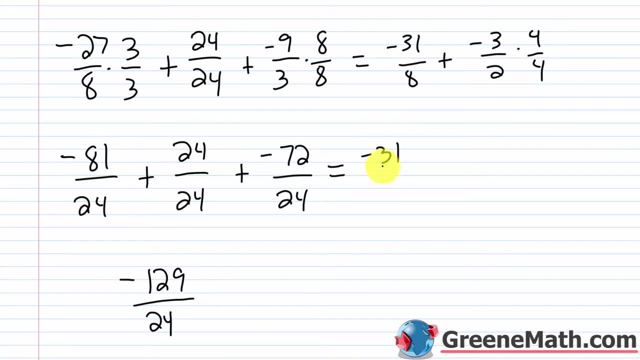 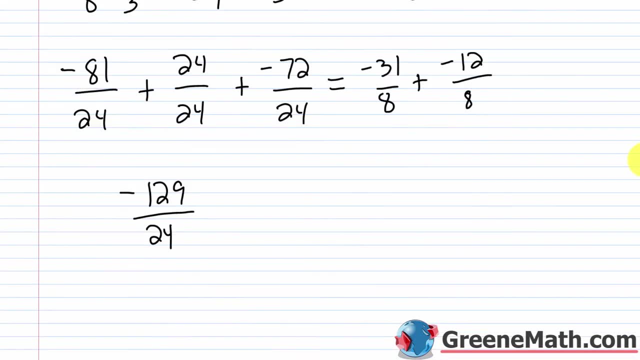 So I just need to multiply this side by 4 over 4 and I'd have negative 31, eighths plus negative 3 times 4 is negative 12 over 2 times 4 is 8.. So negative 31 plus negative 12 is going to be: 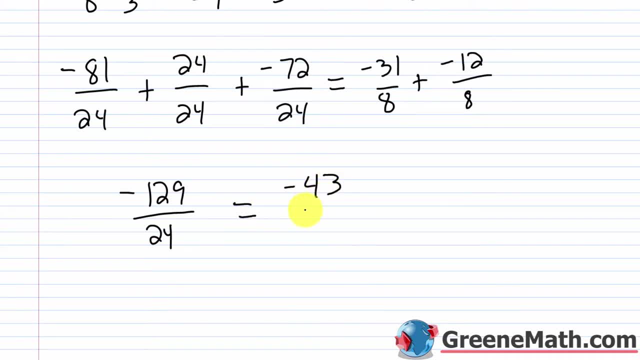 negative 43.. So we'll have equals negative 43 eighths. So a lot of you at this point will stop and go. okay, I got the wrong answer. What happened? Always make sure that when you get fractions, they're reduced to their lowest terms or they're simplified. 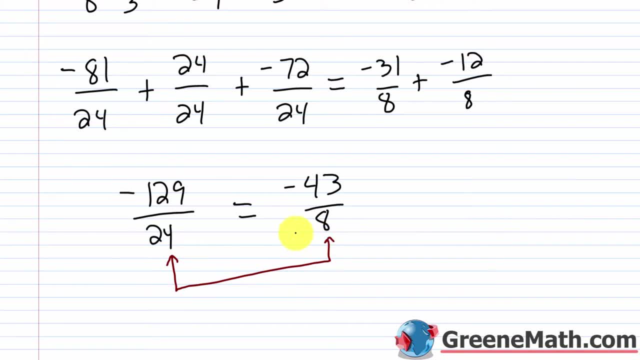 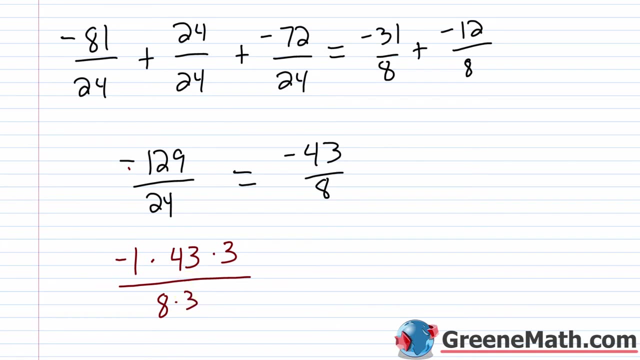 These fractions are the same. The one on the left is just not simplified. If I think about negative 129, I can write this as negative 1 times 43 times 3.. I can write 24 as 8 times 3.. And we can see that we can cancel this 3 with this 3.. 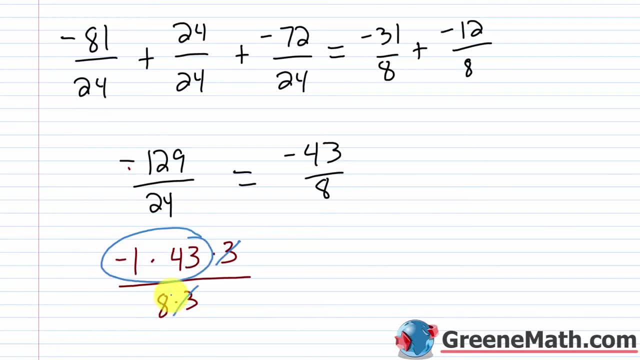 And I'm left with negative 1 times 43 or negative 43 over 8.. That's what I have over here: Negative 43 over 8. And you can't simplify that any further. Right on either side It doesn't matter, because you got the same number on either side. But 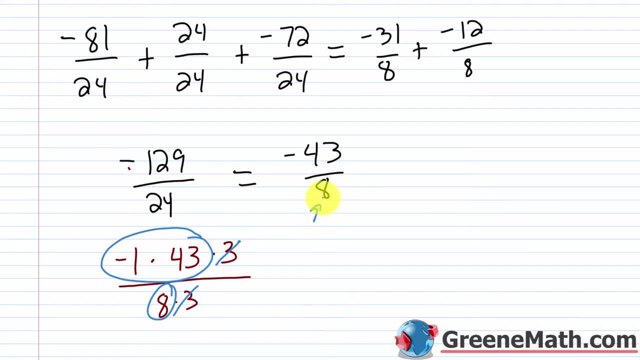 if you wanted to think: okay, well, can I simplify this further just for the sake of completeness? You can't right, because 8 is 2 times 2 times 2 and negative 43 is not divisible by 2.. So you'll end up with negative 43 eighths equals negative 43 eighths, And so you know your solution, which. 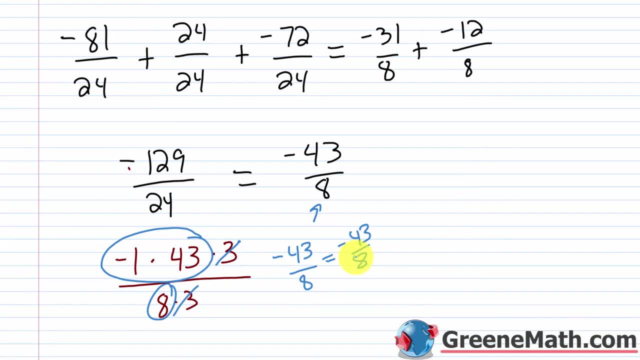 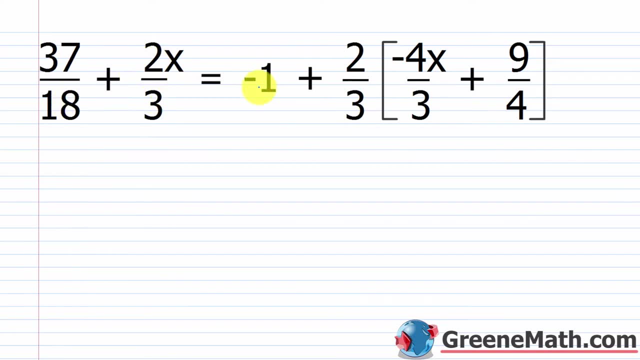 we found was: x equals negative 9 fourths is correct. All right, let's take a look at another type of problem you're going to come across. Two-thirds x equals negative 1 plus two-thirds times this quantity negative. four-thirds x plus 9 fourths. If I begin my problem the normal way, If I say okay, what's the LCD of all the fractions? 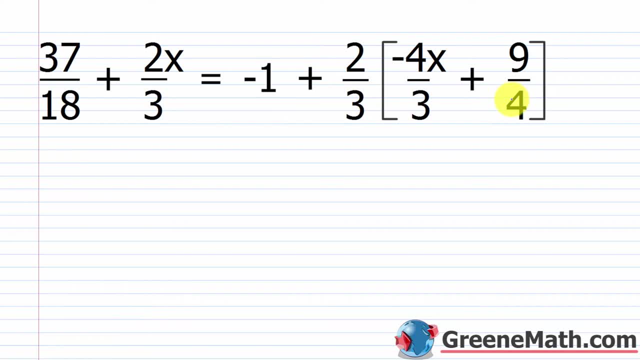 involved And I go to multiply it. It's not going to clear all the fractions right away. What you need to do is use your distributive property first. So if you come across a problem where you have fractions that are inside of a set of parentheses, 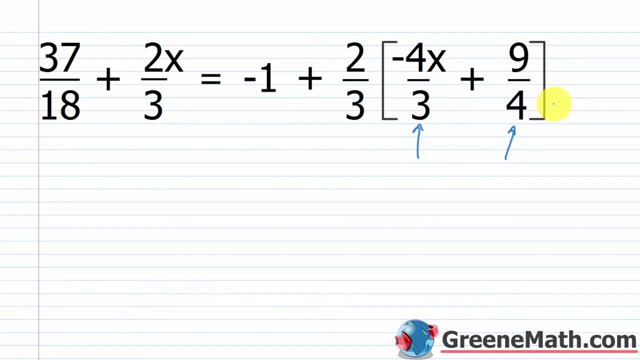 Or a set of brackets. Use the distributive property first and simplify, So what I want to do. So I have 37 eighteenths over here, Plus two-thirds x equals negative 1 plus I'm going to remove the brackets. Two-thirds times negative. four-thirds x: I'm going to have two-thirds times negative. 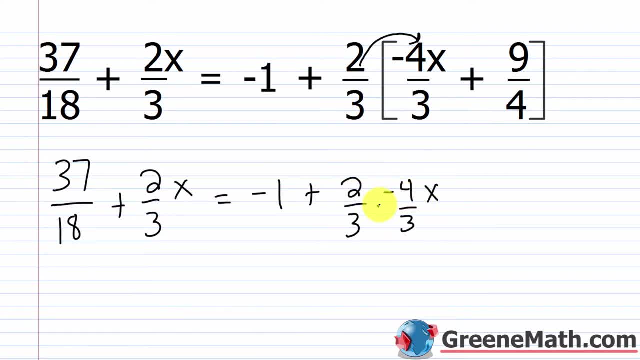 four-thirds x. So 2 times negative, 4 is negative 8.. 3 times 3 is 9.. So this would be negative 8. so I'm going to put minus minus 8, ninths times x, And then again two-thirds times 9, fourths. 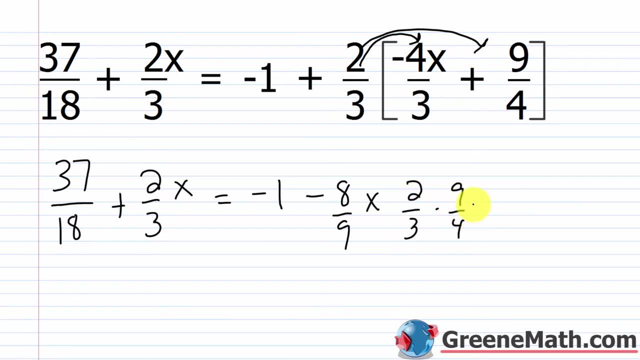 So two-thirds times 9 fourths, And what I can go ahead and do is cancel this with this. That'll give me a 3.. Cancel this with this, And that'll give me a 2.. So this is canceled completely. It's. 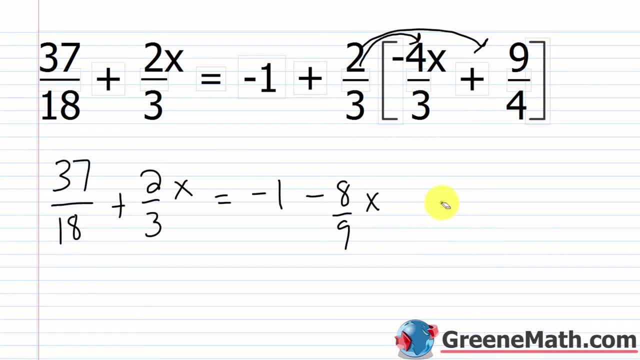 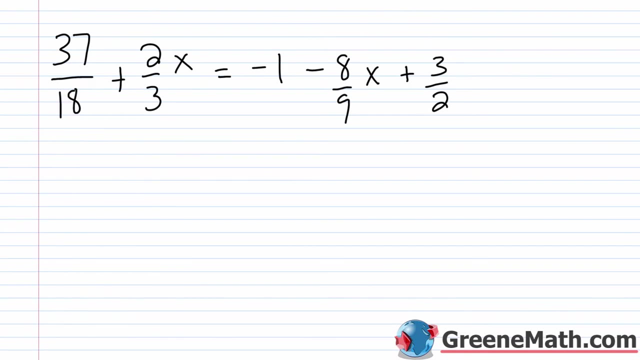 just a 1., And so I'll have three halves there. So this will be plus plus three halves, Okay. So once you've done that, go ahead and think about: okay, what's the LCD now? So I have 18.. I have 3., I have 9. And I have 2.. And at this point in your math career you should be able to. 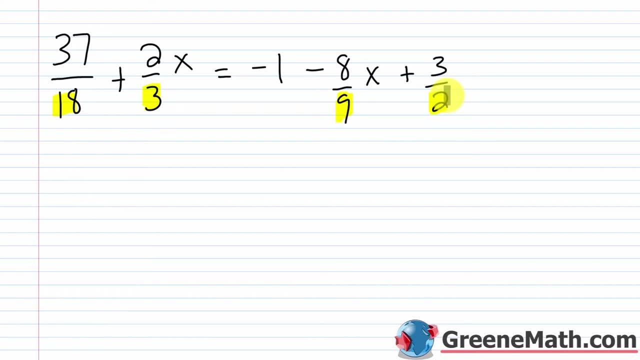 kind of look at that and say, okay, I know the LCD is 18.. Right, So I know most of you can do that If you can't again take the steps. So LCM of 2,, 3,, 9, and 18.. So I know that 2 doesn't factor. 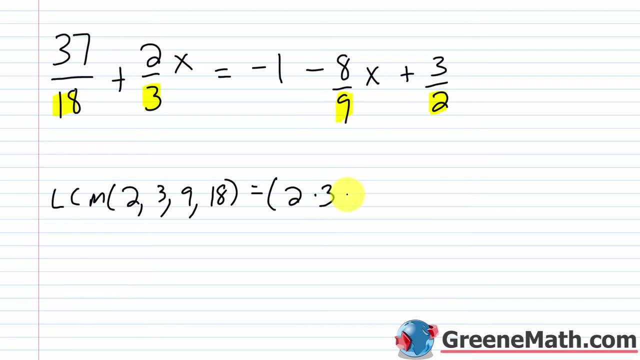 I know that 3 doesn't factor. 9 is 3 times 3.. So I'm only going to put one more copy of 3 in there, because 9 is 3 times 3.. I only want the largest number of repeats to go in. 18 is 2, which I 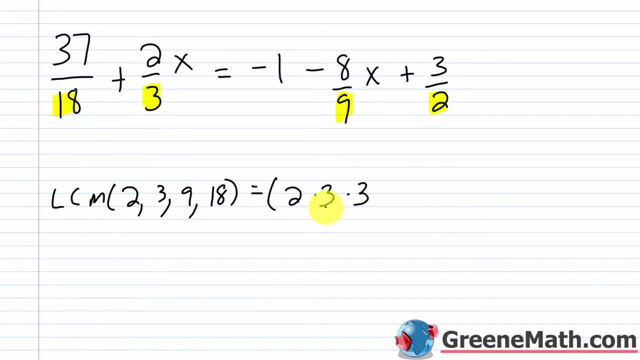 already have in there. times 3, which is already in there. times 3 again. You could think about it as 2 times 9 or, you know, 3 times 6.. However you want to do it, it's going to break down into 2 times 3. 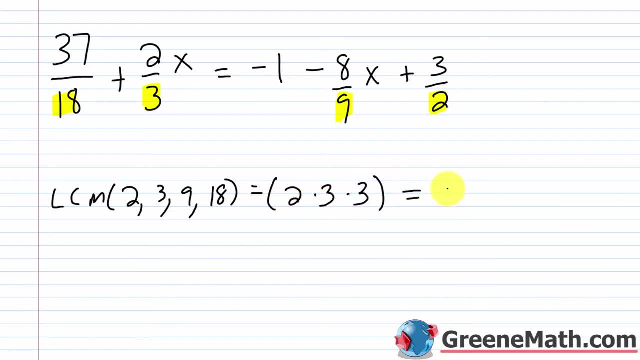 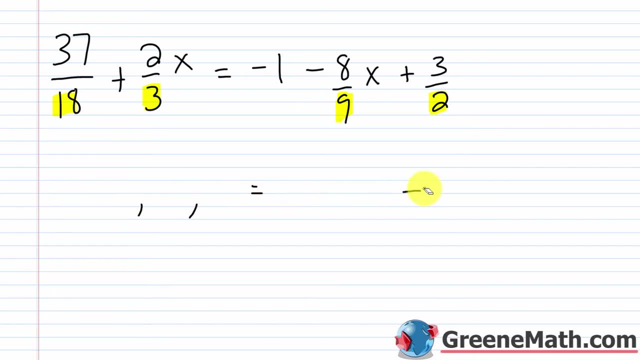 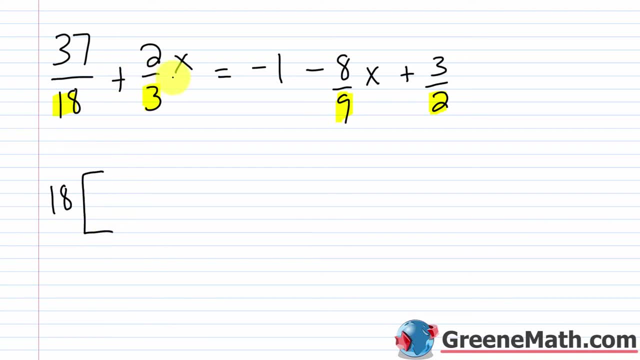 18.. Again, you want to use brackets or parentheses? Make sure that you multiply each term by 18.. All right, So over here on the left, if I do 18 times 37, eighteenths, we know that 18 would cancel with 18.. All right, So this would just be. 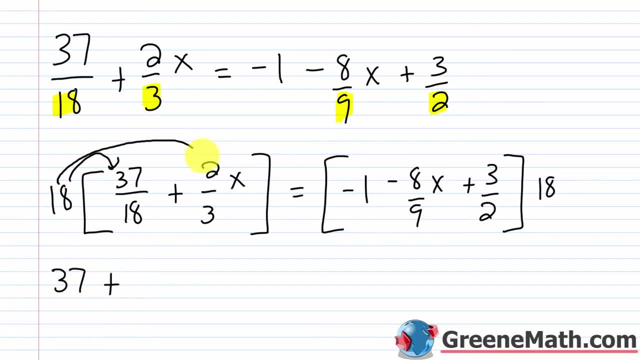 37. Then plus we have 18 times two. thirds x 18 would cancel with 3, giving me a 6.. 6 times 2 is 12.. So this would be 12x And this equals over here 18 times negative. 1 is negative 18. Over. 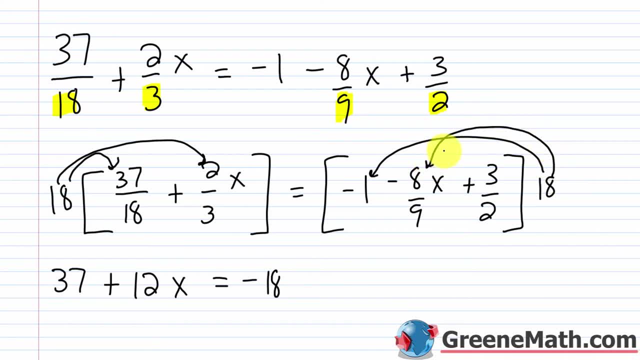 here 18 times negative, 8, ninths. Think about 18, canceling with 9 and giving me a 2.. 2 times negative 8 is negative 16.. So this would be negative 16 times that variable x, Then plus, Lastly, I have 18 times 3, halves 18. 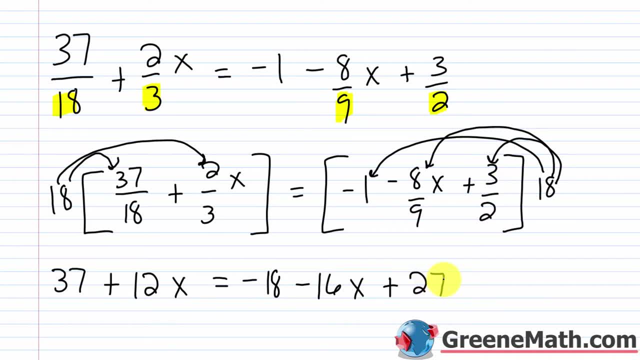 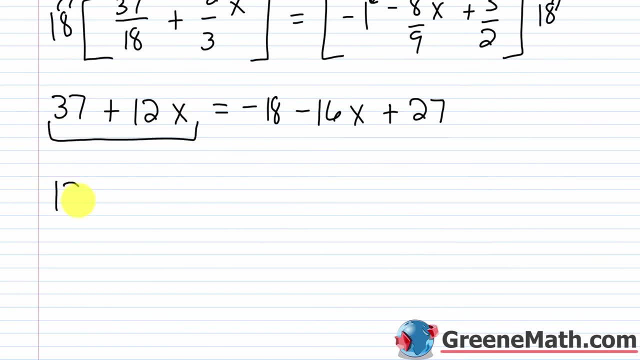 would cancel with 2 and give me a 9.. 9 times 3 is 27.. Okay, Now we just simplify. So I can't do anything to the left. I'm just going to copy that down. So 12x plus 37. I'm just going to reverse. 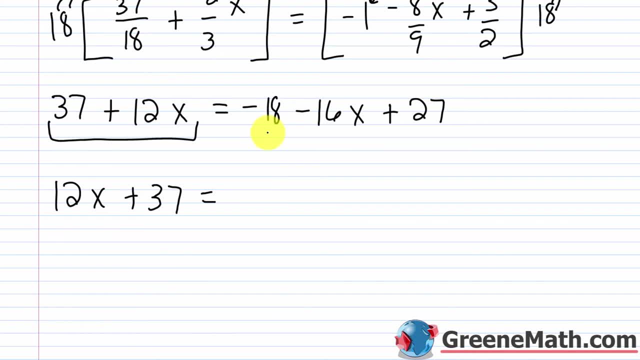 the order On the right. I can simplify because I can add negative 18 and 27.. That's going to give me positive 9. So I'd have negative 16x. I'm just going to copy that down. So I'm just going to. 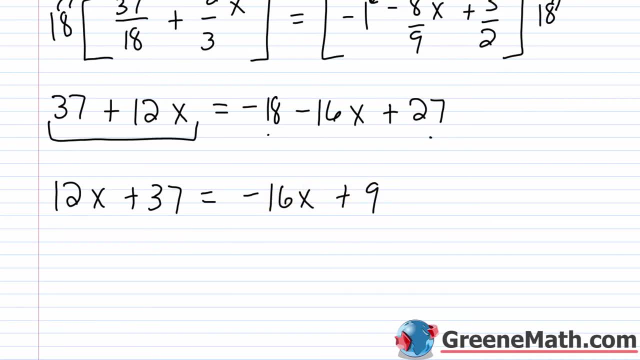 add negative 16x plus 9.. I want all my variable terms on one side of the equation. So because I have one there and one here, I always like my variable on the left. I'm going to move that guy over there. So I'm going to add 16x to both sides of the equation. So that's going to go away 12x. 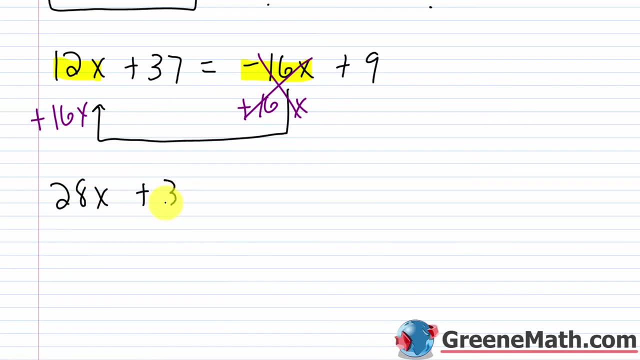 plus 16x is 28x. So plus 37 equals 9.. I'm going to get my variable term by itself on the left. So that means I'm going to be subtracting away the 37. From both sides of the equation. So that's gone. So I'll have 28x equals What is 9 minus 37?? 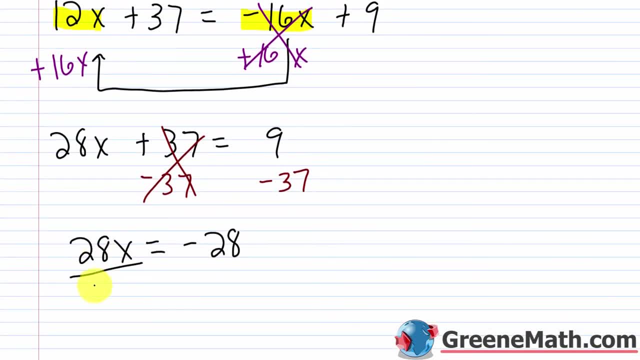 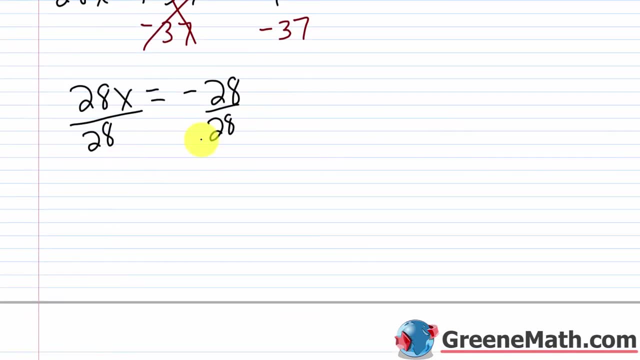 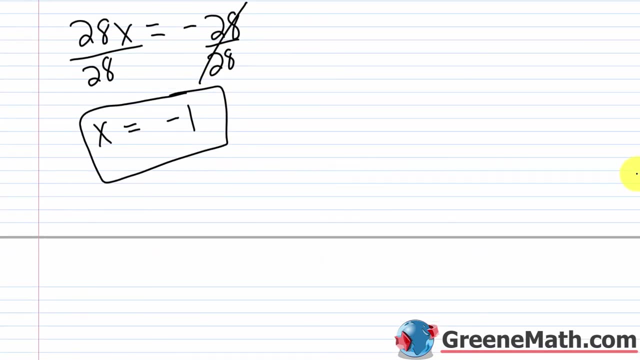 That's going to be negative 28. And we divide both sides of the equation by 28.. The coefficient of x, in order to isolate the variable completely, And I'm going to have x, is equal to negative 1.. Okay, X is equal to negative 1.. All right, So we could erase all this and check. 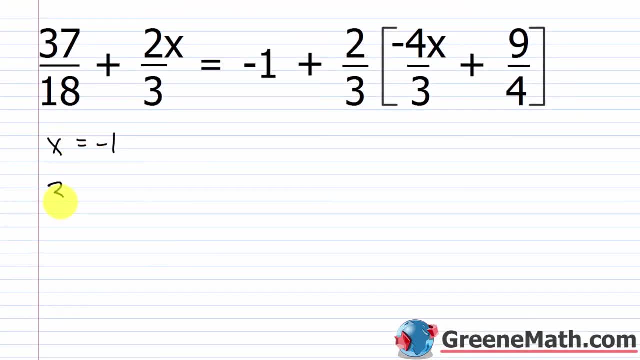 So x is equal to negative 1.. All right, So we could erase all this and check. So x is equal to x. Again equals negative 1.. So we'd have 37 18ths plus 2 times negative 1, which is just. 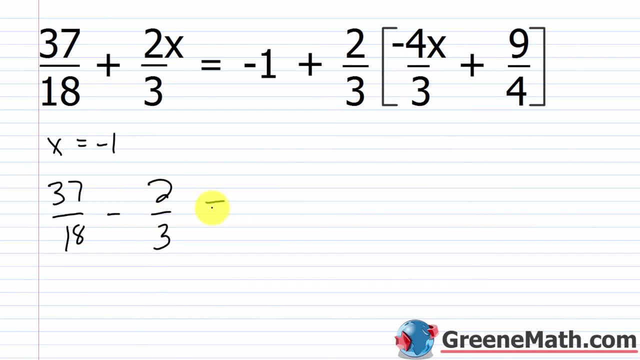 negative 2.. So I'm just going to write minus 2 thirds, And this is equal to negative 1 plus 2 thirds times this quantity, We'll have negative 4 times negative 1. So that's positive 4 over 3. 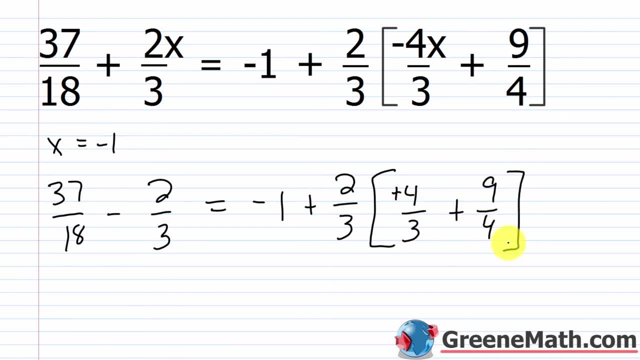 plus 9 fourths. So on the left side, I just multiply this by 6 over 6. And I'll have a common denominator Right. So I'm going to have negative 1 plus 2 times negative 1.. So that's. 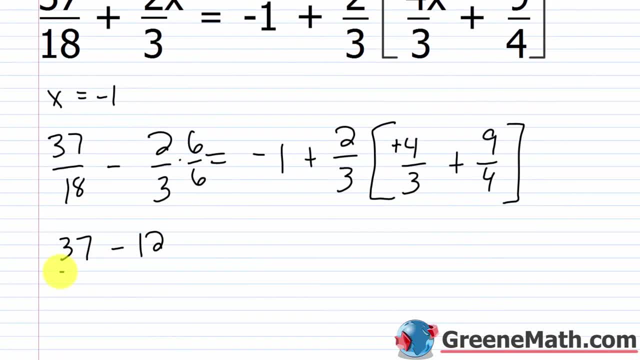 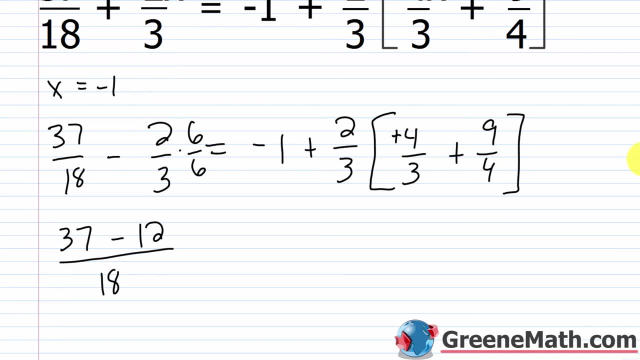 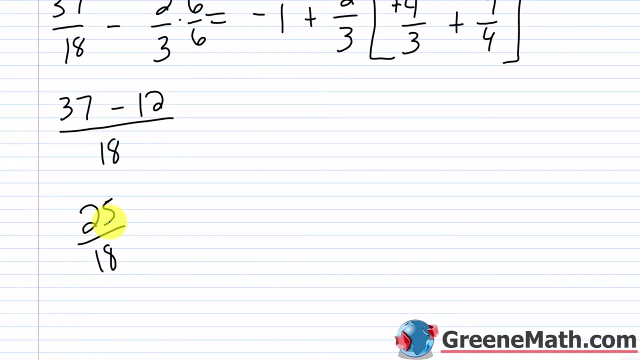 So I'd have: 37 minus 2 times 6 is 12 over the common denominator of 18.. 37 minus 12 is 25.. So this would be 25 over 18.. 25 over 18.. And 25 is 5 times 5.. 18, we know, is 2 times 3 times 3.. 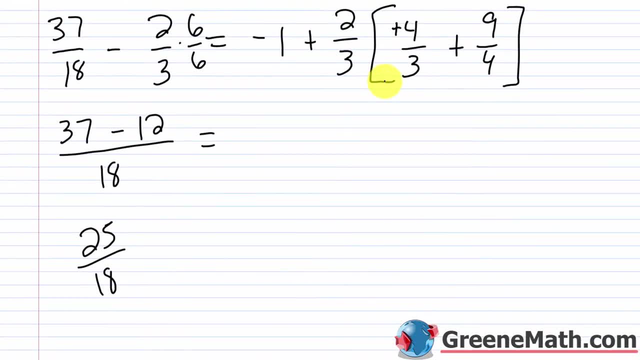 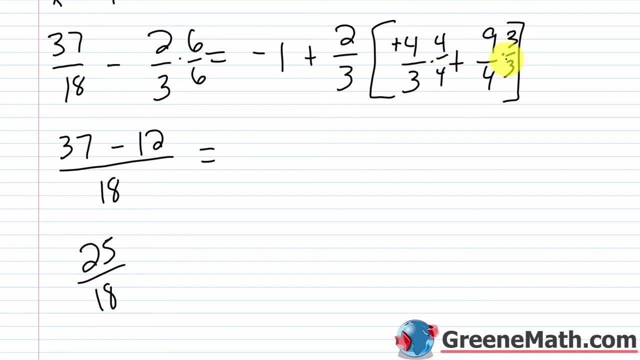 So really we can't make that any more simple Over here. if I think about 4 thirds plus 9 fourths, I'd multiply this by 4 over 4.. I multiply this by 3 over 3. And so negative 1 plus 2 thirds times 4 times 4 is 16 over 12. plus 9 times 3 is 27 over 12.. 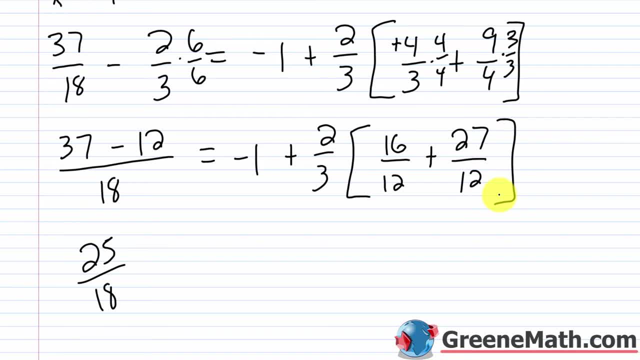 And 16 plus 27 would be 43. So I'd have 43 twelfths. So let me just erase this and write 43 twelfths. So if I'm multiplying here, this is going to cancel with this and give me a 6.. 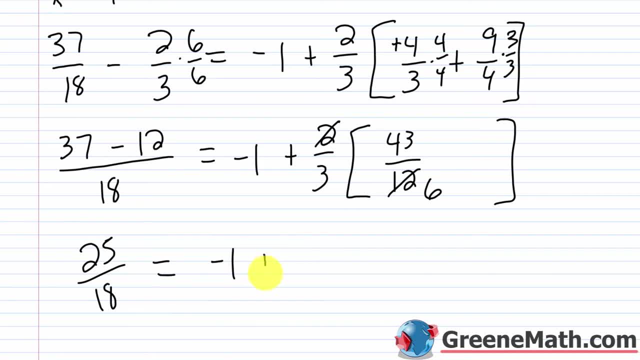 And so what I'm going to have is negative 1 plus I'll have 1 times 43, or 43 over 3 times 6 or 18.. So to get a common denominator here, I'm going to write this negative 1 as negative 18 over 18.. So we just need to think about what is. 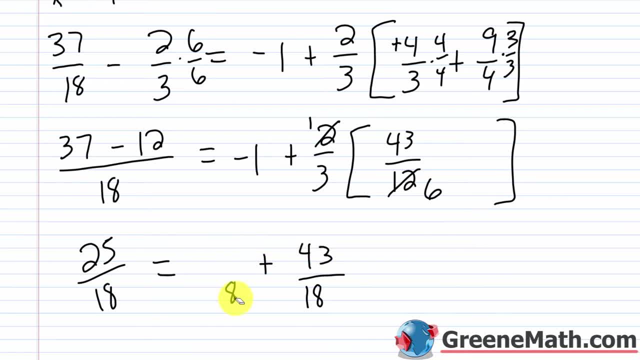 43 minus 18?? Well, that's 25, right? So this becomes 25 eighteenths, just like on the left side of the equation, And so we know that our solution- x equals negative 1, is correct. So let's. 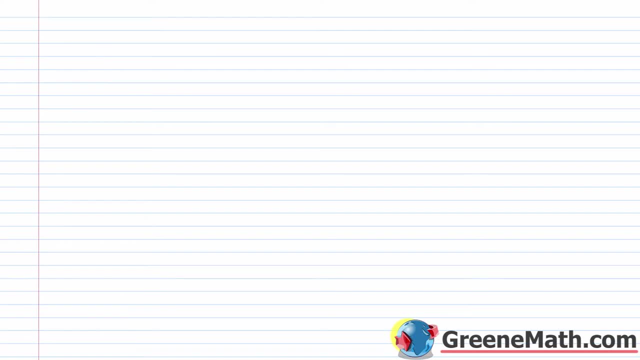 talk a little bit about when your equation has decimals in it. So in most cases, you're using calculators on your exams or your homework, and working with decimals when you have a calculator is not any more difficult. So this is just something I'm teaching as a matter of completeness. You do need to know how to do it, because you 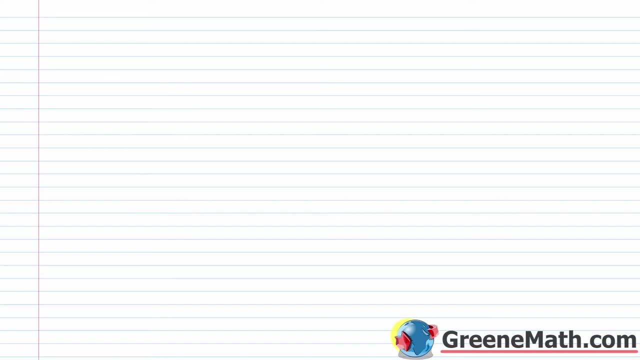 might be asked for it on a test, but I don't think it would actually save you any time, especially if you're working with a calculator. But if you're faced with decimals, I just want you to think back to when we learned that if you multiply by 10, or 10 raised to 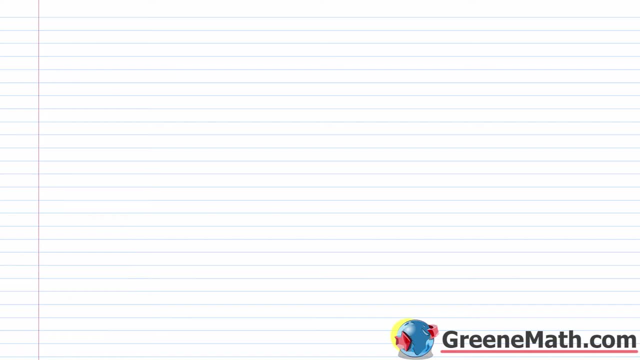 a whole number, That is one. We're going to move our decimal point one place to the right for every zero in our power of 10.. So, for example, let's say I have the number six and I multiply by 100.. Well, I. 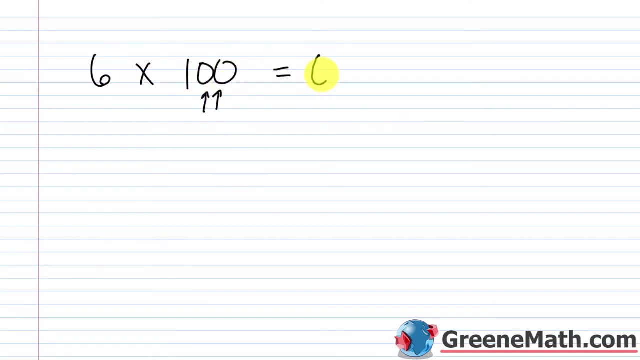 have two zeros in this power of 10.. And so I take six, I write a decimal point after six, because you can always write six as six point zero, And then I can move the decimal point two places to the right to get my answer, because I have two zeros in that power of. 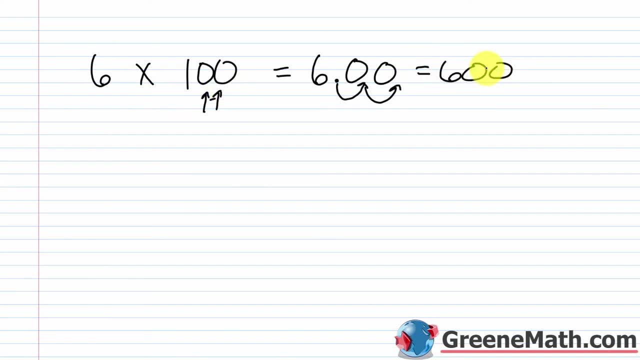 10.. So this is really 600, right, We know that six times a hundred is 600.. We also could write a hundred as 10 to the second power And kind of the shortcut is the: look at the exponent there and say, okay, I have two places that I'm going to move my decimal point to. 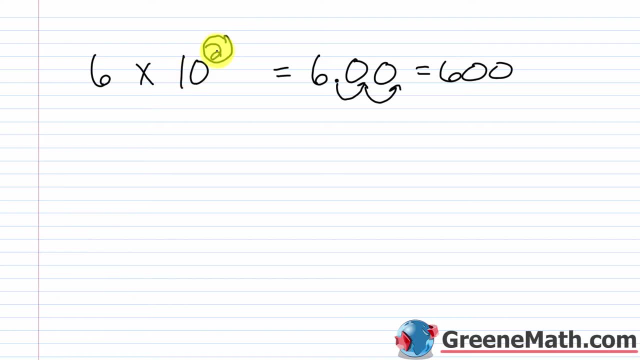 the right, Because if you have a 10 raised to the power of two, it's going to be a one, followed by two zeros, And once you get good at this, you can be very, very quick with these calculations. So let's say I had three times 10 to the fourth power. I see that there's 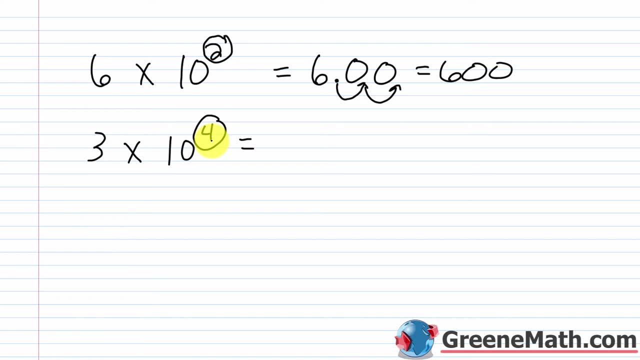 a four here. Here's my exponent. That means that I would have a one followed by four zeros. right? That's what 10 to the fourth is. So this would be a three. put my decimal point down, and I'm going to move that decimal point four places to the right, because there's a four there. 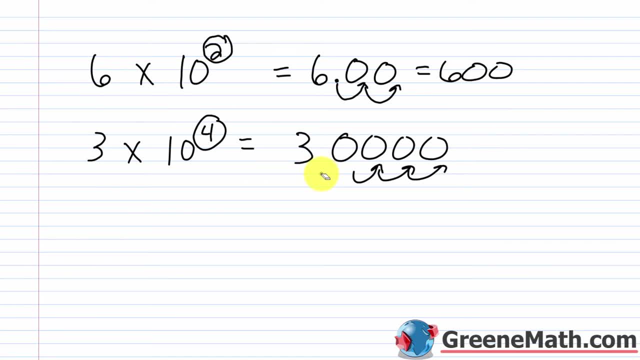 So one, two, three, four, and I'm going to end up with 30,000, right, Because 10 to the fourth power, 10 to the fourth power again, is a one, followed by four zeros. So one, two. 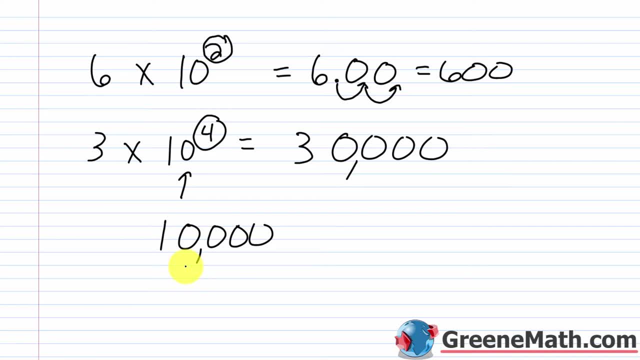 three, four or 10,000.. And you can kind of mentally see that three times 10,000 is 30,000.. It's pretty easy to do. So if we do this and we involve kind of some decimals, we can kind 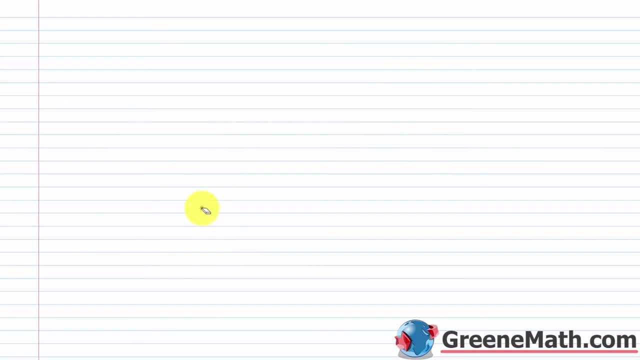 of use the same principle to clear the decimals. So if we have 6.32, and I want to make this into a whole number, meaning I don't want to see this decimal point anymore- I have one, two decimal places here. All I need to do is multiply it by a number that has a one. 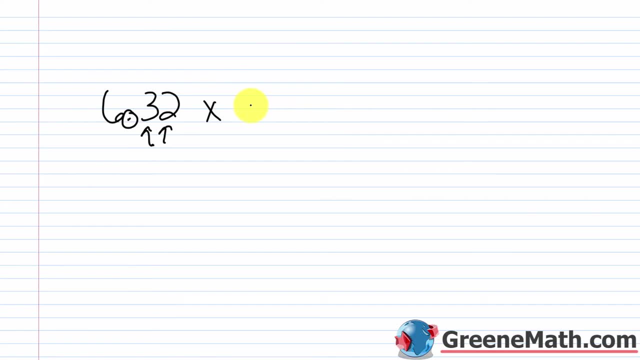 followed by two zeros, right, So I'd multiply it by 100.. And squared, sometimes, 100.. So this would be equal to 632, right, Because this would go one, two places to the right. So, essentially, what's going to end up happening is we're. 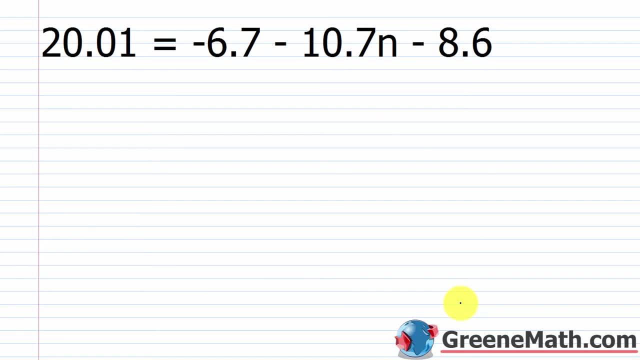 going to look at our equation and we're going to see the largest number of decimal places between everything involved. So we're then going to multiply both sides of the equation by a power of 10. that will clear that decimal. So you want to clear the largest number of. 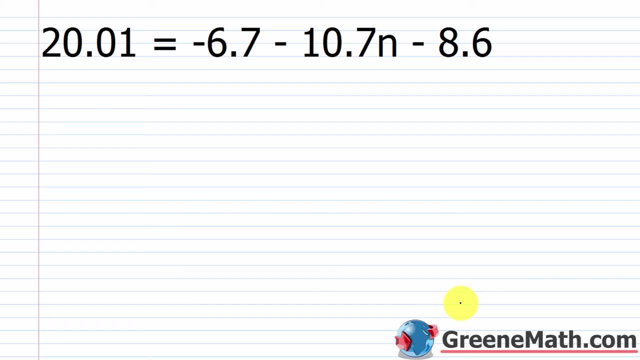 decimal places. So if the largest number of decimal places you have is three, then you're going to multiply by 1,000,. right, It's a power of 10 that has a one followed by three zeros. And if you clear the one that has the largest number of decimal places, 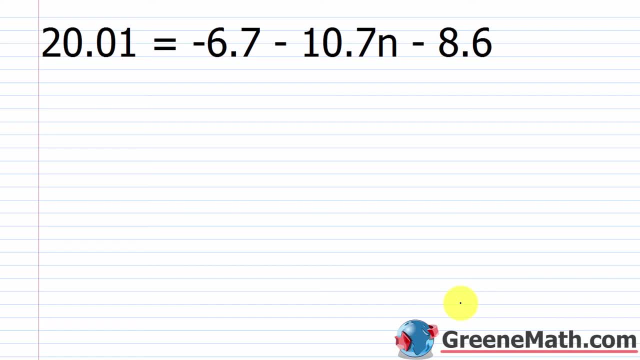 you're going to clear all of them, All right. So let's take a look at: 20.01 equals negative 6.7 minus 10.7n minus 8.6.. I'm going to look through this equation. I have one, two decimal. 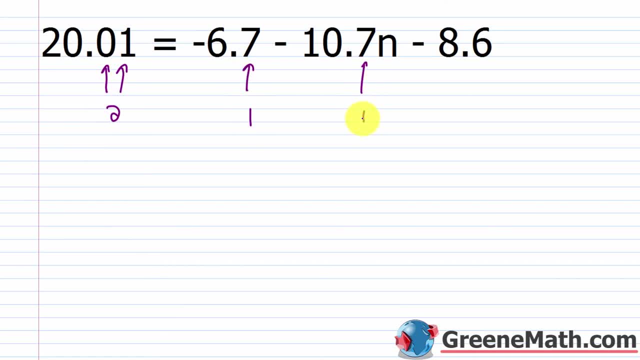 places here. I have one decimal place here, one here and one here, So the largest number of decimal places between any of these numbers involved would be two. Now, in order to clear the equation of decimals, I need to multiply by a power of 10. that will allow me to move. 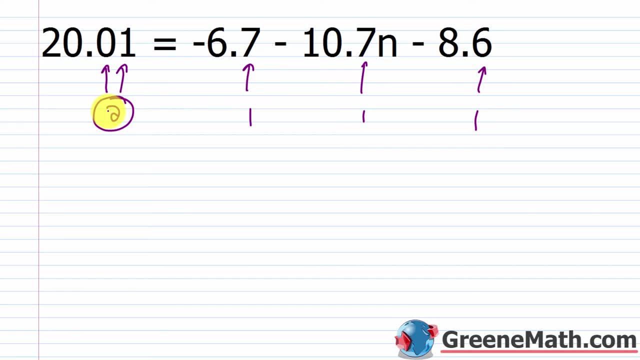 all the decimal points in the equation, two places to the right. So to do that, you're going to multiply by 100.. Okay, Just think about. okay, I need two zeros in the power of 10.. So that's 10 squared or 100.. So again, I'm going to use parentheses or brackets to 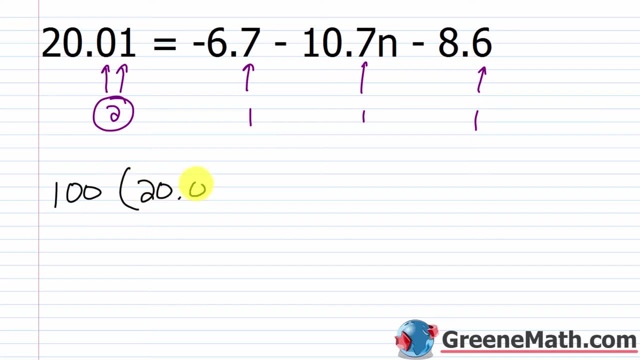 put 100 outside, 20.01 equals- and I have 100 outside of here too- negative 6.7 minus 10.7n minus 8.6.. Very, very easy. Now we're just going to use our distributive property. So 100 times 20.01,. 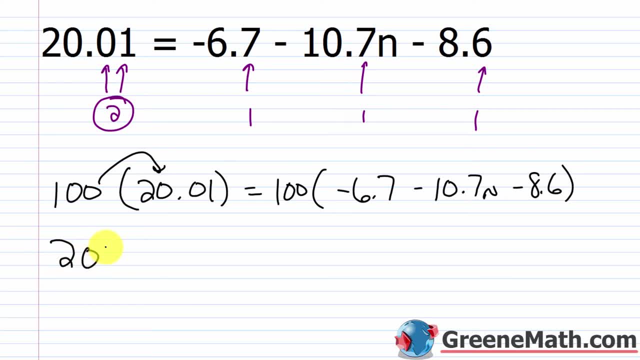 again move your decimal point two places to the right, So this would be 2001.. This is equal to, over here, 100 times negative 6.7.. You'll have a negative, You'll have six, You'll have six. This is going to go one, So I'll have a seven. and then one more place to the 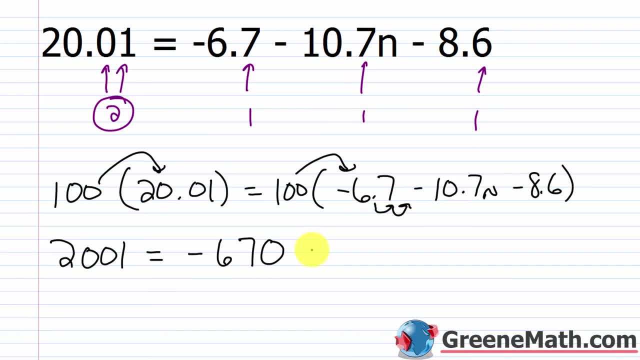 right And so a zero. so negative 670.. And then minus, here we have 10.7n, So I'm going to have 10.. This is going to go one place to the right. That's going to be a seven. one more place. 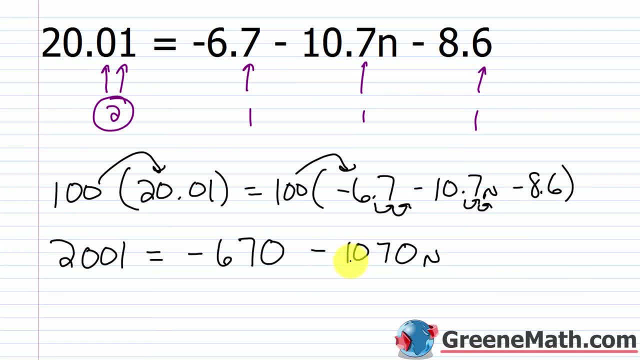 to the right. That's going to be a zero, and then my n, so that's minus 1,070 n And then minus, here We have 8.6.. So that's going to be 860, right, This is going to go one. 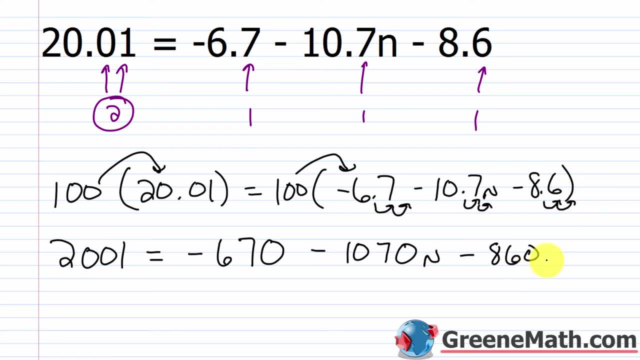 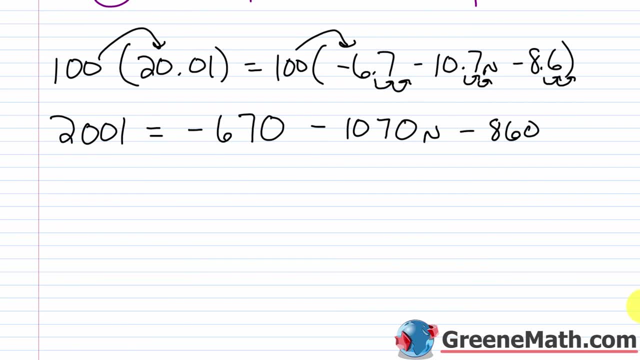 two places to the right here and then right there. so we have a transformed equation now that doesn't have any decimals involved and again you just go through after you have this and do your regular procedure. so i would combine like terms here: on the right: negative 670 minus 860 is negative 1530. so 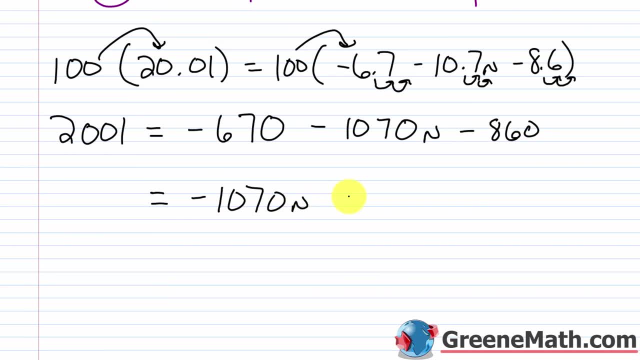 this will be negative 1070 n and then minus 1530, and this is equal to over here on the left we have 2001. so i still want to isolate my variable term and to do that, i'm going to add 1530 to both. 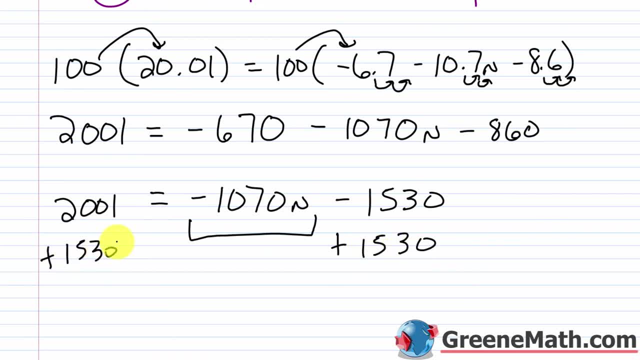 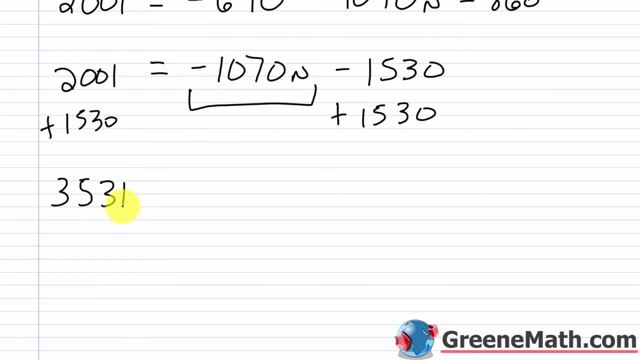 sides of the equation. and so 2001 plus 1530 is 3531 and this equals negative 1070 n. all right now to get n by itself. i just divide both sides of the equation by the coefficient. so divide by negative 1070, divide by 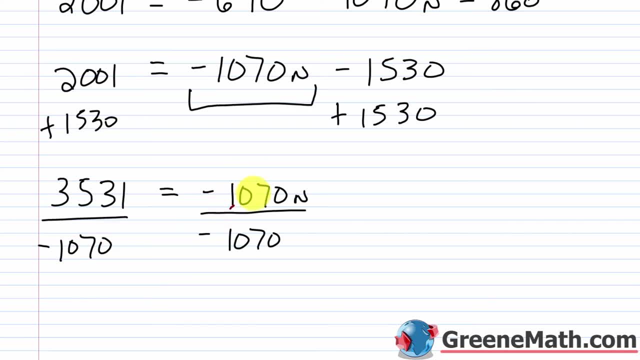 negative 1070 and this will cancel with this. and then 3531 divided by negative 1070 is going to give me negative 3.3, so i get negative 3.3 equals n. now notice how i wrote it like that, versus as a fraction. you can do either, because we're working with decimals. i chose to write: 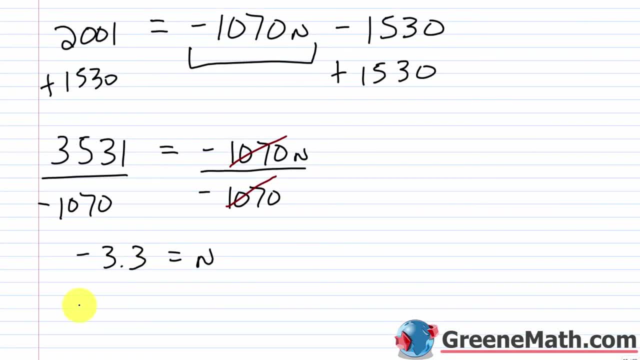 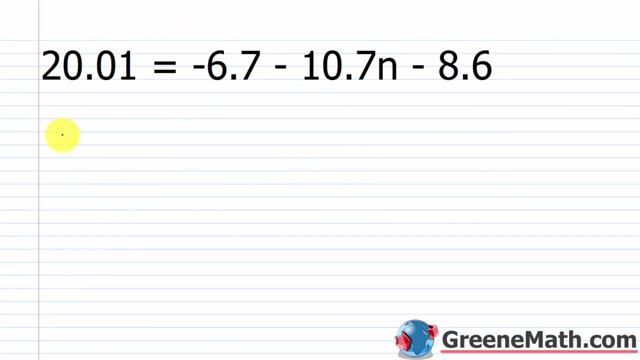 this as a decimal. you can do either one, it does not matter. so i'm going to rewrite this as n equals negative 3.3 and we're going to go back up to the top and check it. okay, so we're going to have n equals negative 3.3 here. so we're going to have: 20.01 is equal to negative 6.7. 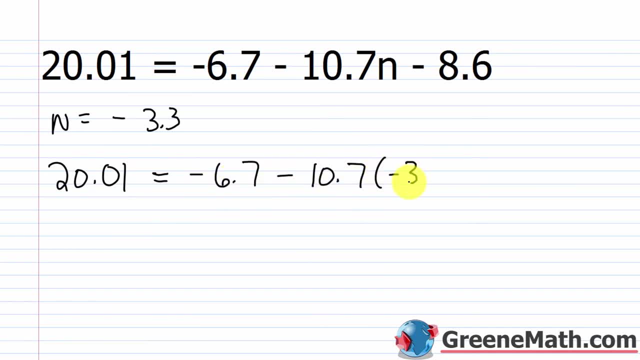 minus 10.7 times again negative 3.3 minus 8.6. okay, so over here on the left, 20.01 is not going to change. don't need to do anything there. on the right, i need to do my multiplication first. what is negative? 10.7 times negative 3.3. 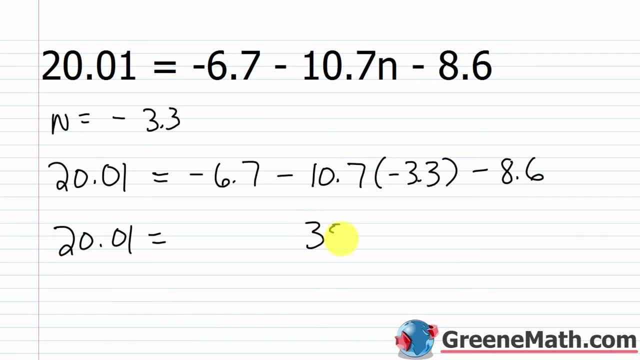 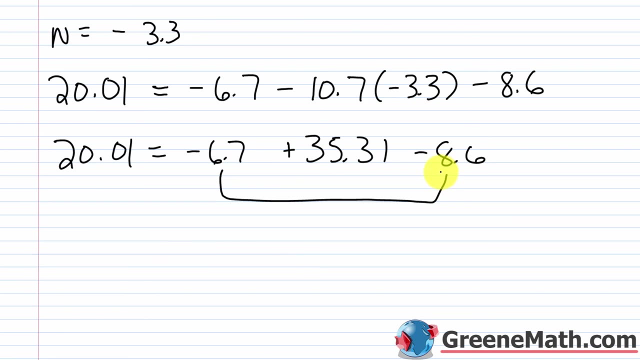 it's going to give me 35.31, 35.31. okay, so now i have negative 6.7 plus 35.31 minus 8.6. so i'm going to add my numbers with like signs first: what is negative: 6.7 minus 8.6. that's going to be negative 15.3. so i'm going to write that. 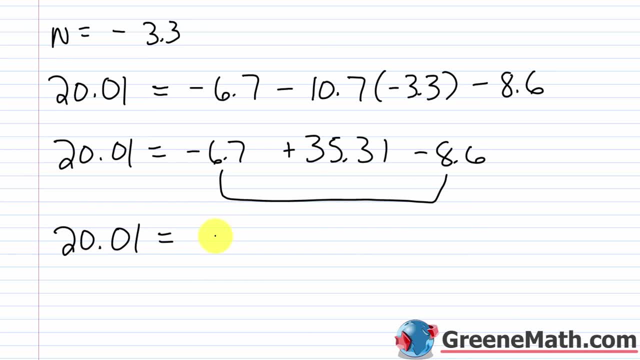 says 20.01 equals negative 15.3 plus 35.31. and now we just need to add over here what is negative: 15.3 plus 35.31. that's going to give me 20.01. so 20.01 equals 20.01, same number on the left and 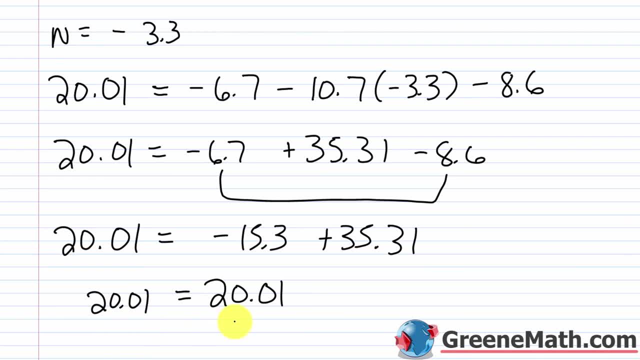 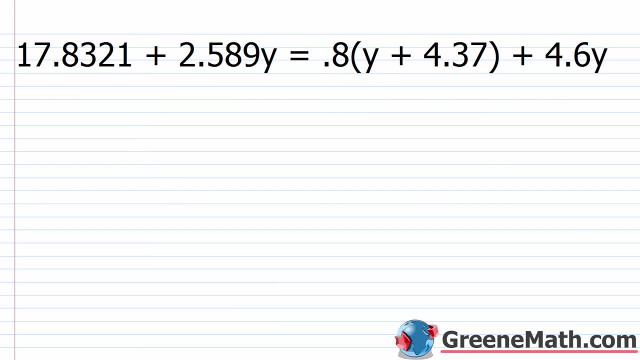 the right. so n equals negative. 3.3 is the correct solution. all right, let's take a look at another one. we have: 17.8321 plus 2.5891 equals 0.8 times the quantity y plus 4.37 plus 4.6 y. now, just like we saw with fractions. 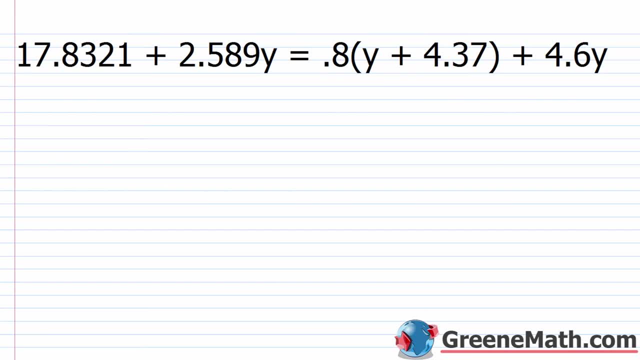 when you're trying to clear decimals, you've got to use your distributive property first if you have decimals inside the parentheses. so 17.8321 plus 2.5891 y equals- distribute this inside here, so 0.8 times y is 0.8 y, and then distribute this inside. 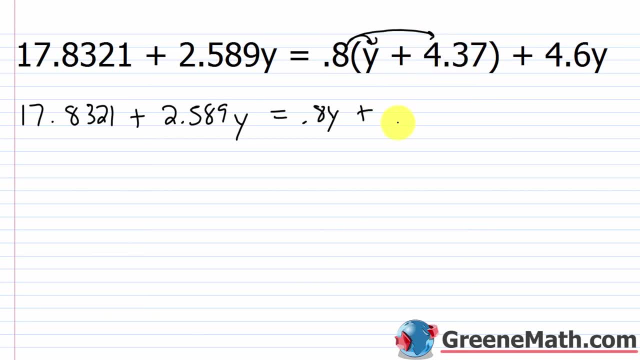 here and then distribute this inside here. so 0.8 times y is 0.8 y, and then distribute this inside here: so plus. so 0.8 times 4.37 is 3.496, so 3.496 plus 4.6 y. so now i'm going to look to. 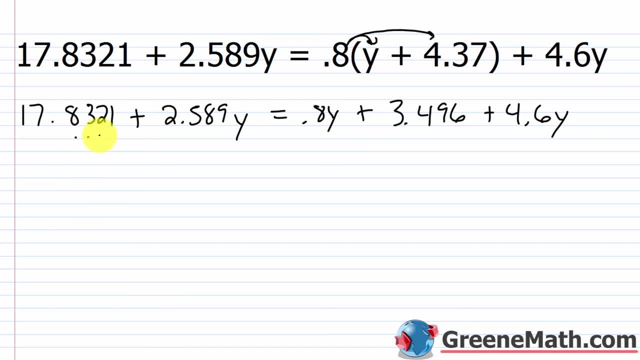 see what number has the highest number of decimal places. i have one, two, three, four here. i have one, two, three here, i have one here, one, two, three here and i have one here. so the highest number of decimal places is four. so that means i need to multiply by a number that has a one followed by a. 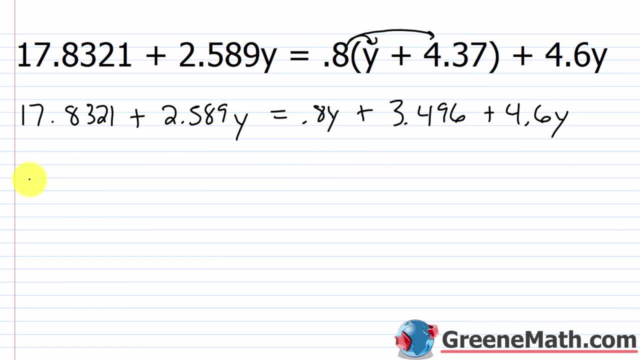 followed by four zeros. so i'm going to multiply both sides of this equation by a one, followed by one, two, three, four zeros for the number 10 000. so i'm gonna have 10 000 times 17.8321 plus 2.589 y. 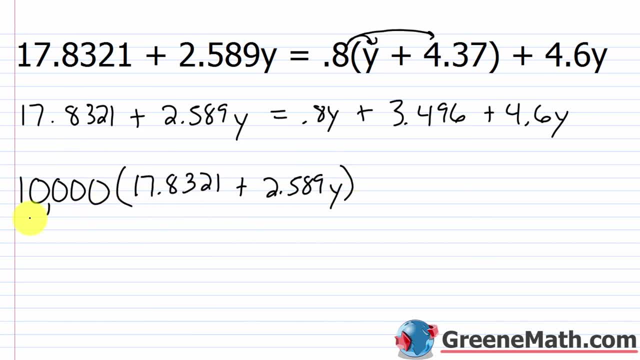 and again, make sure to put this inside of parentheses- you're really multiplying 10 000 by each of these numbers. you can't make the mistake of just multiplying it by 17.8321. it's also got to be multiplied by 2.589- y as well, okay. so over here i'm going to have 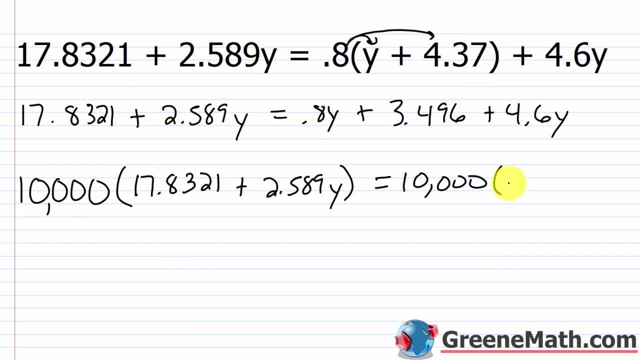 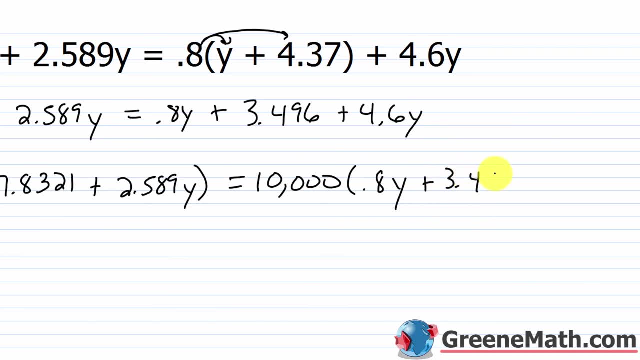 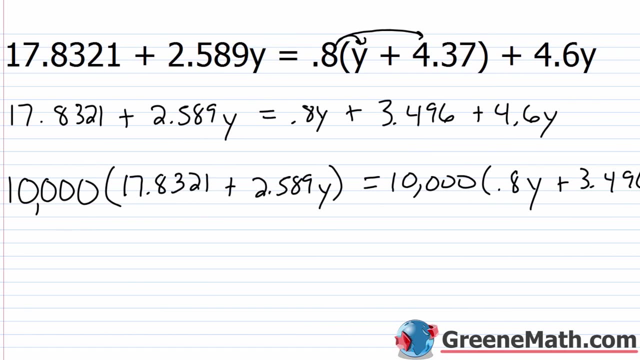 10 000, also multiplied by- and i'm going to put this off the screen for a minute- so we'll have 0.8 y plus 3.496 plus 4.6 y, again inside of parentheses. okay, so starting over here on the left, if i multiply 10 000 times 17.8321, 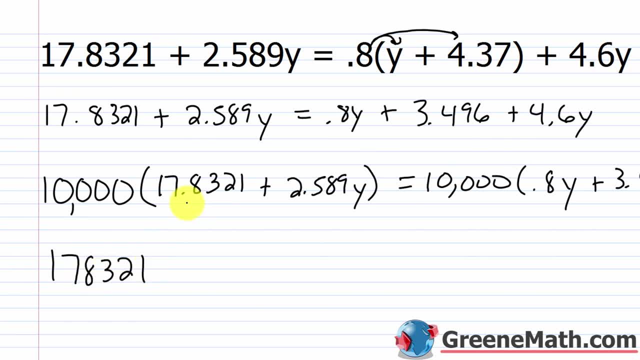 it's going to be one, seven, eight, three, two, one right. this will go four places to the right, and so i end up with 178, 321. so then plus now, if i multiply 10, 000 by 2.589 y, i'm basically going to have two, five, eight, nine, and then a zero at the end. again, this goes four. 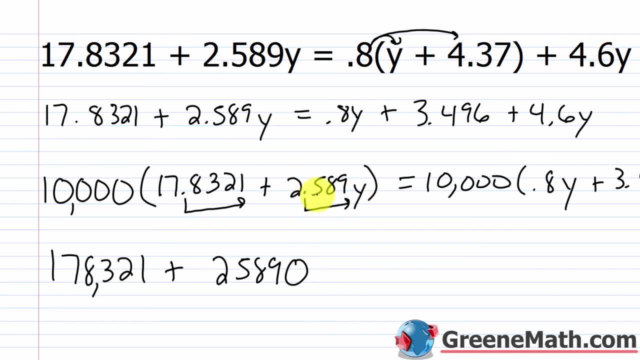 places to the right, and so it would pass the nine and then go one more right. so that's why i have zero here. we'll go one, two, three, four, and then i have ten thousand and i'm going to have two, three, four places to the right. So that ends up giving me 25,890, and then times the variable y. 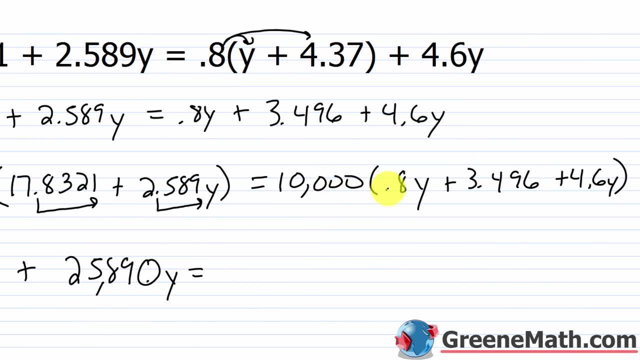 And then over here on the right, I have 10,000 times 0.8y, So I have 0.8, and this goes four places to the right. It's going to go one, two, three, four, So that's going to be 8,000.. Then 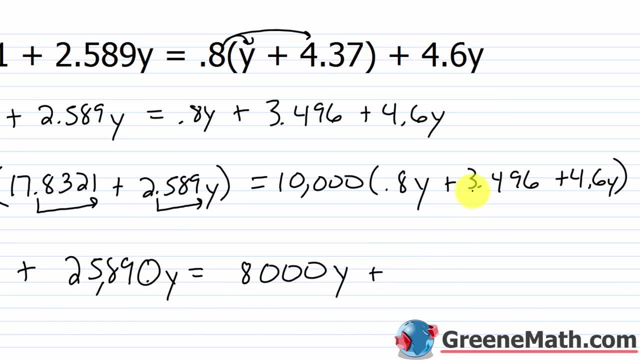 again times the variable y, Then plus over here I have 3.496.. So this is going to go four places to the right. So it's going to pass the six by one more place. So I'm going to need to write 3,. 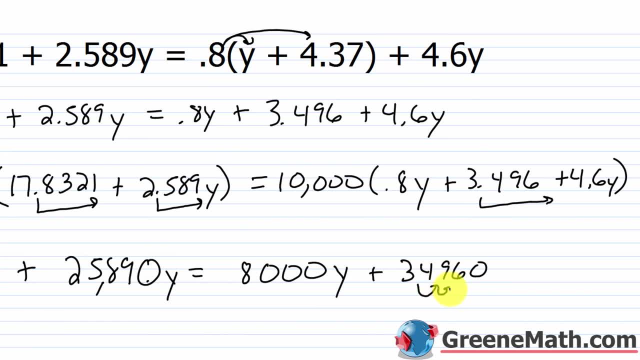 4, 9,, 6, 0.. This is going to go one, two, three, four places to the right, And then plus we have 4.6y, So 10,000 times 4.6,. we think about 46 here And I'm going to need to put three more zeros. One. 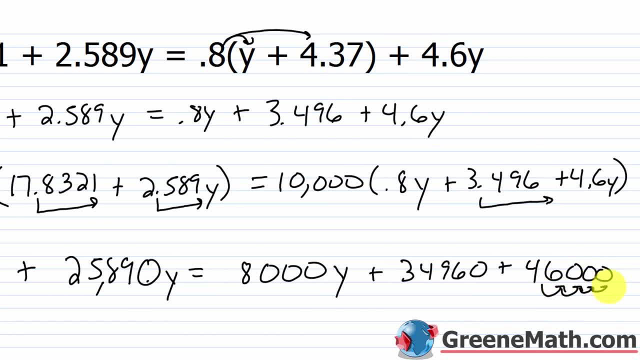 two, three. This is going to go one, two, three, four places to the right, And then don't forget the y, And then we have 4.6y, So that's going to pass the six by one more place. So I'm going to. 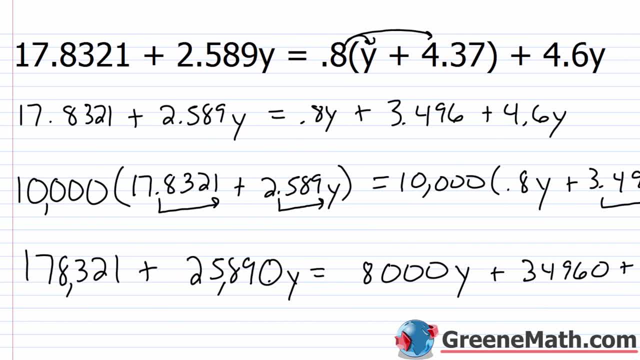 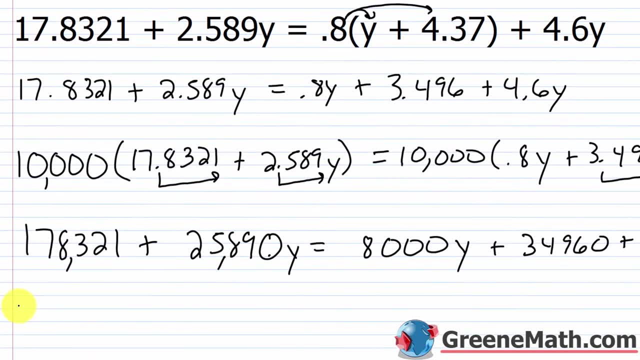 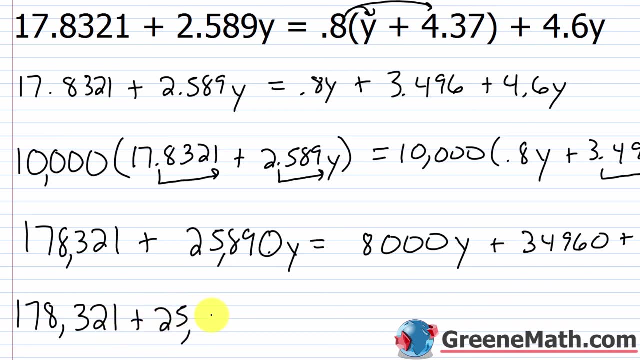 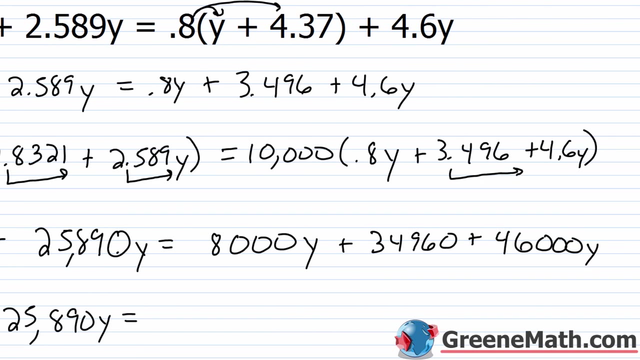 have our transformed equation. Unfortunately it's so big it doesn't fit on the screen. But we go through the same process On the left. I can't simplify any more, So I'm just going to write: 178,321 plus 25,890y. This is equal to over here on the right. I can combine like terms. 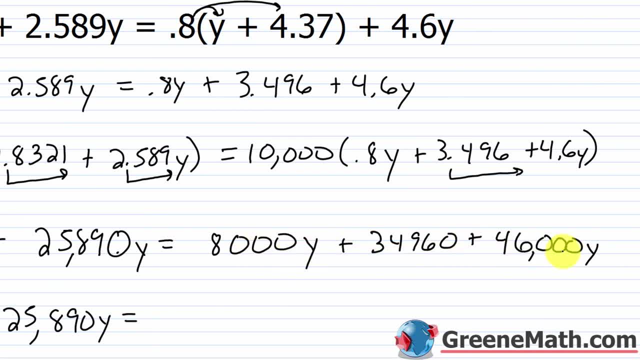 And I need to put a comma in there. I have 8,000y plus 46.. 6,000y, That's going to give me 54,000y, Then plus- and I put a comma in here- 34,960.. 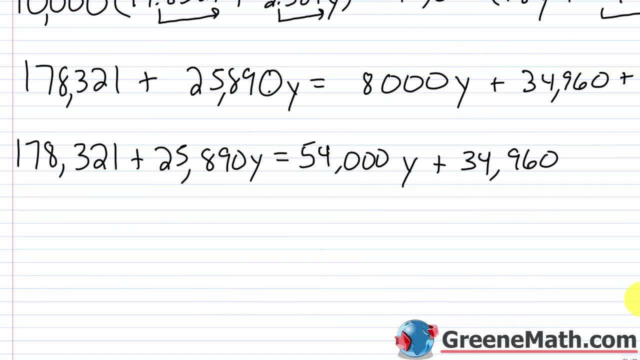 So again, I want all my variable terms on one side of the equation, And so I like my variable term to be on the left. I like my number to be on the right, So I'm going to go ahead and subtract 54,000y. 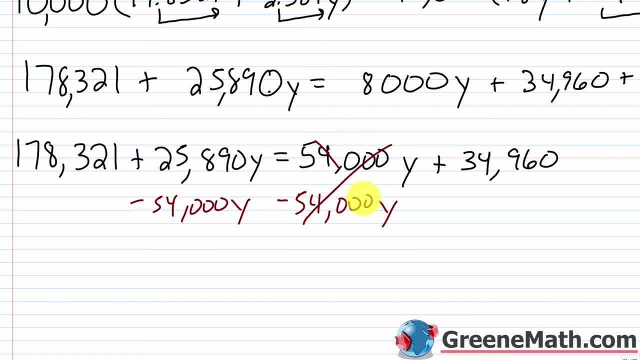 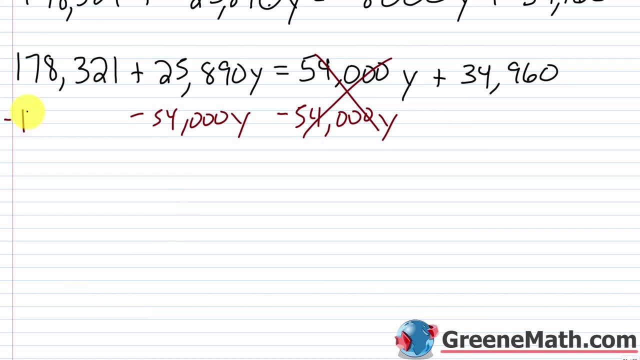 From both sides of the equation. that's going to go away, And just to save a little time, I'm going to simultaneously subtract 178,321 from both sides of the equation. So why am I doing that? Well, what's going to end up happening is I'm going to have a variable term. 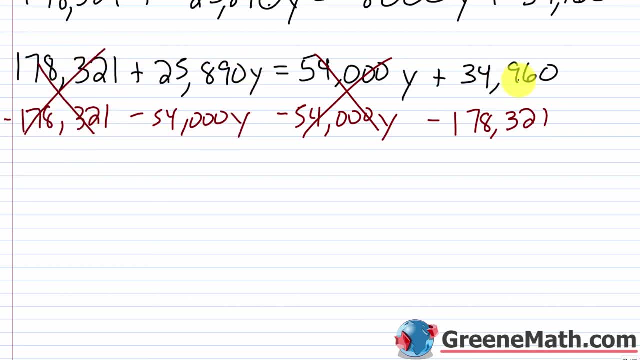 on this side. This is gone And I'm just going to have a number on the right side. All right, So what is 25,890 minus 54,000?? That's going to be negative, Negative- 28,110.. And then y, And this is equal to what is 34,960 minus 178,321..